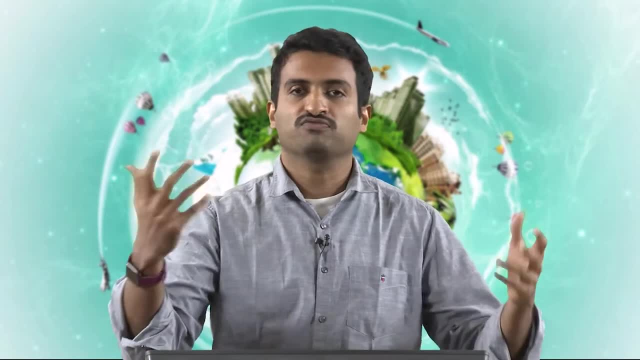 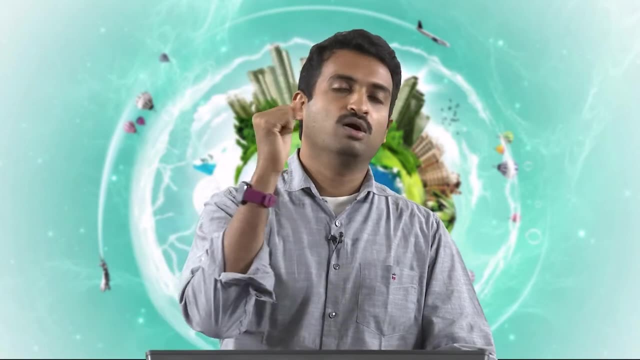 So that is not going to be feasible. And also providing oxygen for a lot of time. So you know that is not an feasible option too, because of the cost. Another aspect is: what do we say? putting in a lot of oxidizing agent? Again, that is going to be costly. 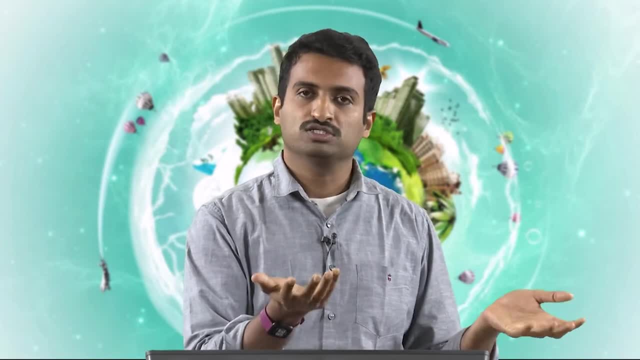 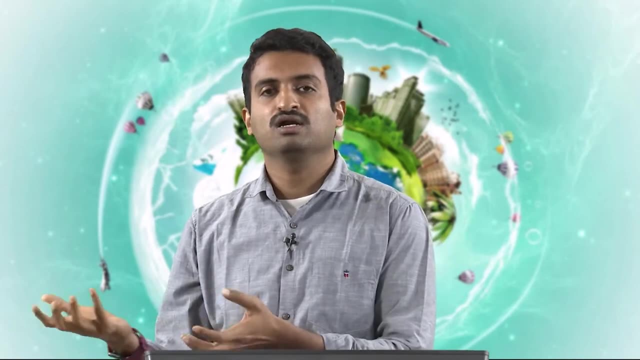 So what are we going to do? We are going to try to mimic what nature typically does. What does nature facilitate? It facilitates microbial growth and these bacteria degrade the relevant wastes or are wastes. So we are going to promote that. How do we promote that? 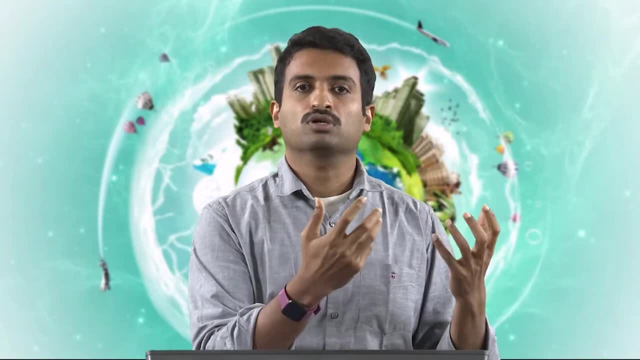 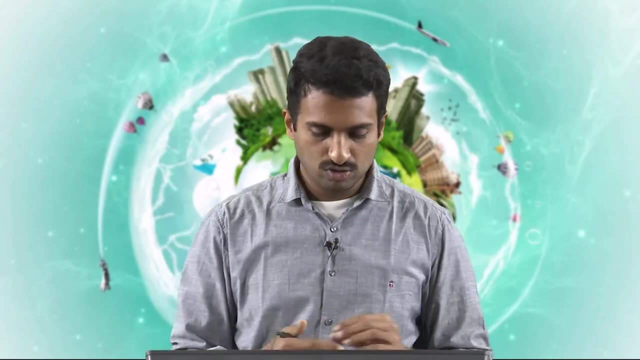 We promote that by Creating conditions that promote bacterial growth and also by increasing the concentration of the microbes in this waste water. So that is what we are going to discuss, or that is the general strategy. So, obviously, for the microbes, what do they need? 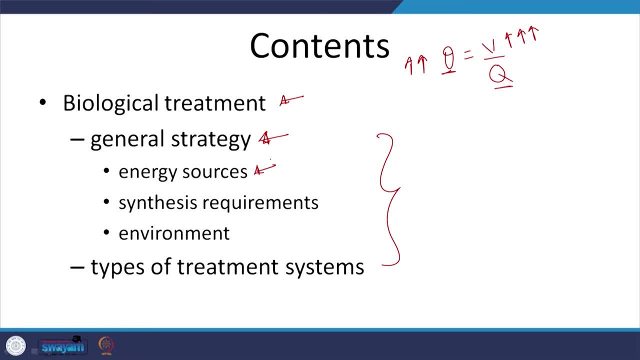 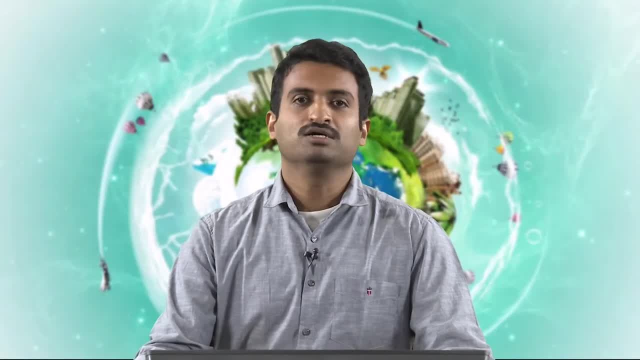 They need sources of energy. Why are they degrading it? Well, they do not have any sense of smell and they do not really like waste water, for due to their, due to its smell or such, They degrade the waste, or are waste, as their food, or consider them as their food, because 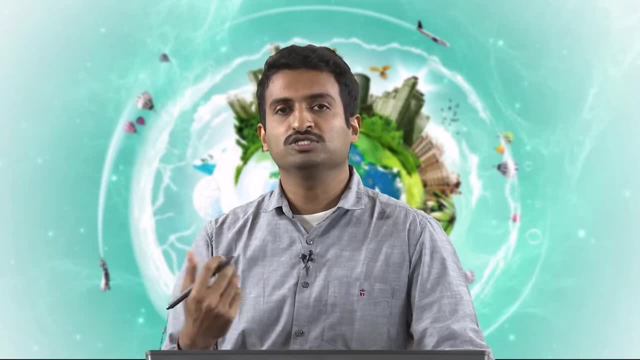 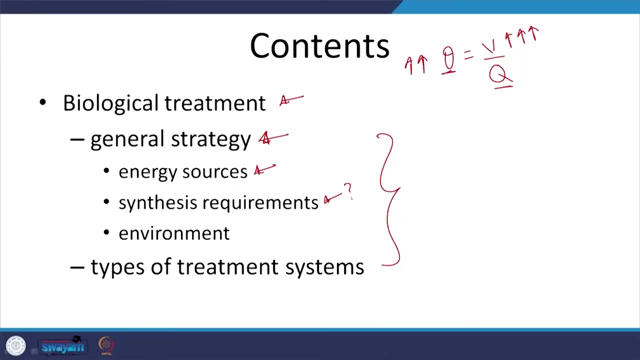 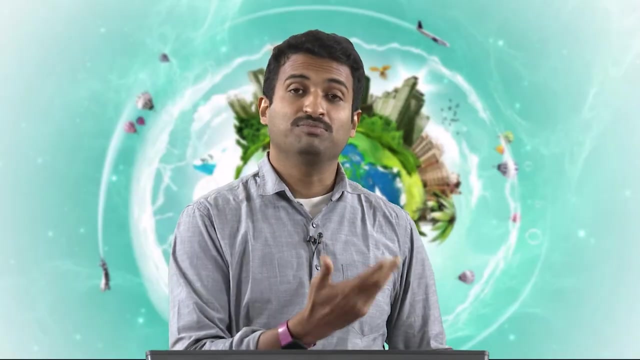 they gain energy from it and then can synthesize new cells. So energy sources to synthesize new cells. what is it that they need? Similar to us, they also need nutrients. we will discuss that. And what about the general environment as in we are or can be stressed? 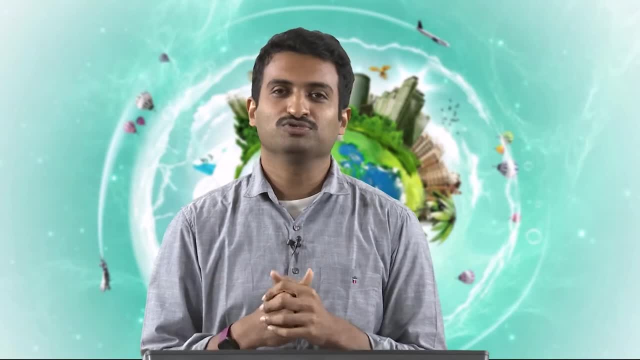 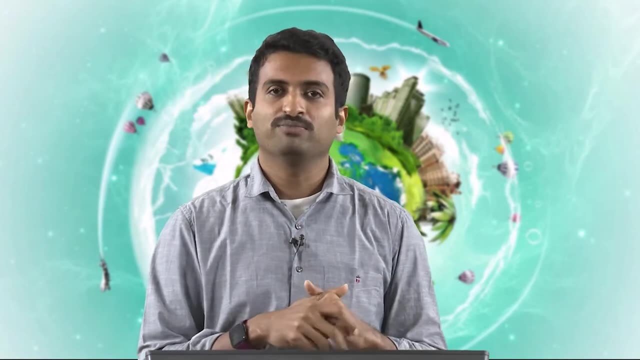 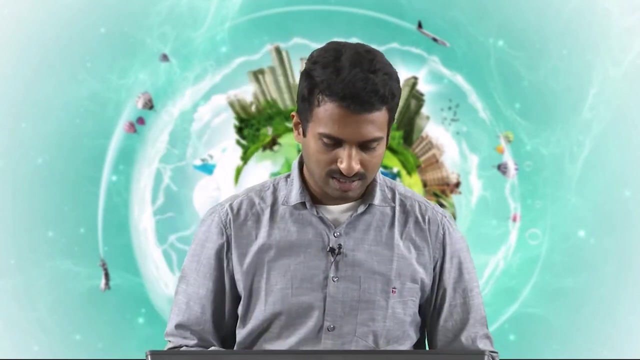 We do have our own peer pressure and relevant issues, work pressure issues, But we are always concerned with the environment: too hot, too cold And these kinds of environmental conditions. Similarly, microbes also have environmental conditions: pH, temperature and so on and so forth. We will look at that. 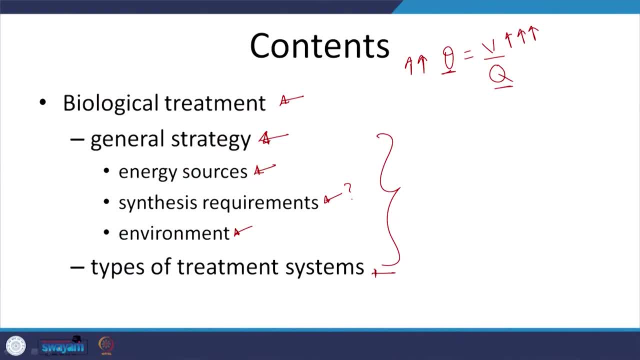 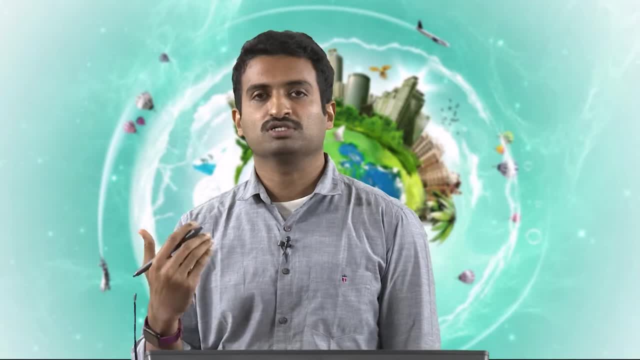 And then, based on these fundamental aspects, there are different modes of treatment systems. We will briefly touch upon some, but discuss activated sludge process in greater detail, because that is the most widely used form of waste water treatment out there. So let us move on here. 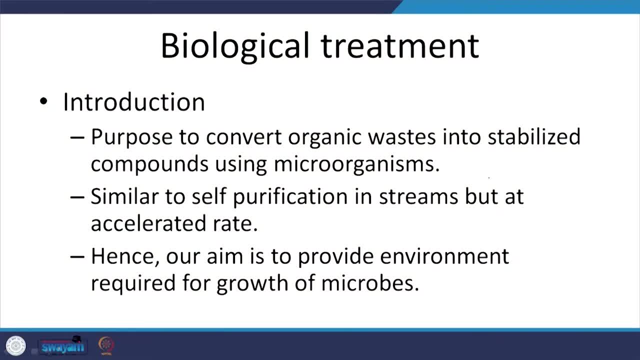 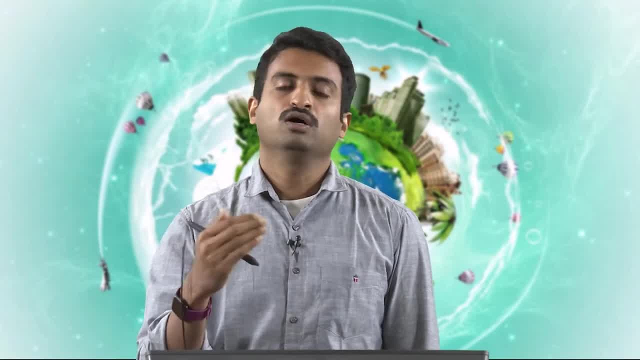 So biological treatment. what are we trying to do? We are trying to? what do we say? see to it that the waste, which if I leave it out there there can lead to septic conditions, smell because of Windows or it is a reduced forms of sulfur like hydrogen sulfide being. 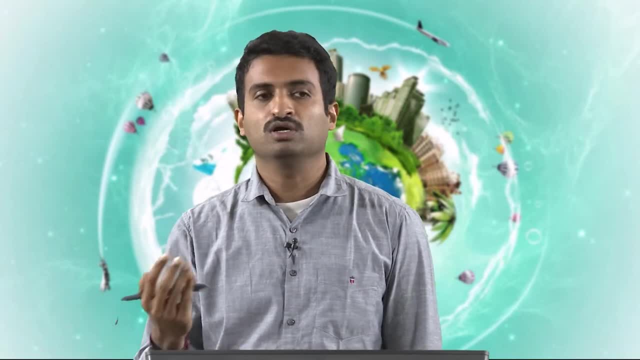 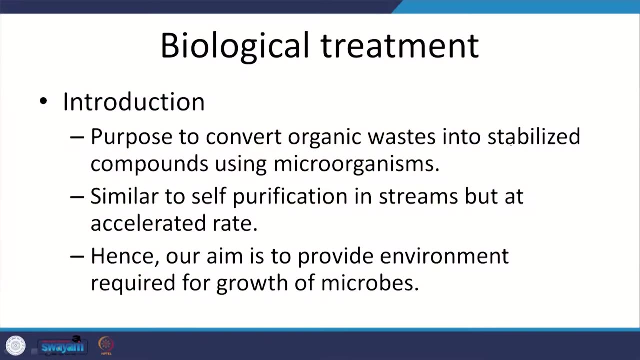 given out. Exposive gas is like methane can be given out, and then you are going to have what do we see? flies and such because of septic conditions and such. so you do not want to have that. you want to have relatively stable PRO compound and we are going to do get to that by using 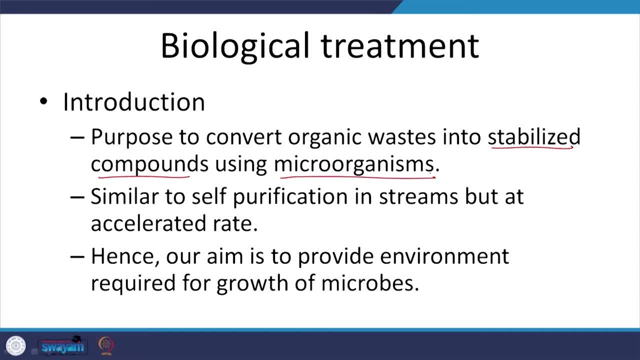 microorganisms which release enzymes, necesarioizes. let us see. Let us see again rami main. Let us say h, Let us say again the melamine main. aim is to degrade the organics, but by promoting the growth of microbes. So 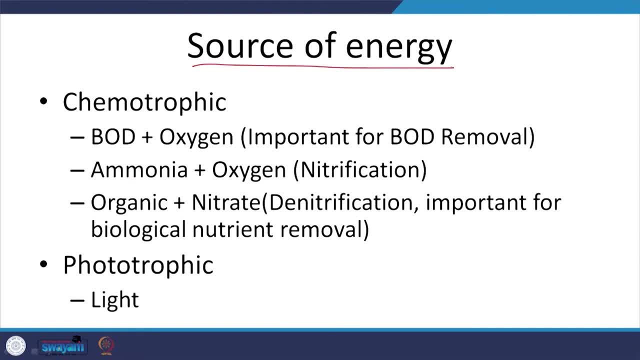 let us move on. So sources of energy, with respect to microbes or microorganisms, we are looking at source of energy or general source of energy, So we can classify them as chemotrophs or chemotrophic and phototrophic- Obviously phototrophic photo, So the source of energy. 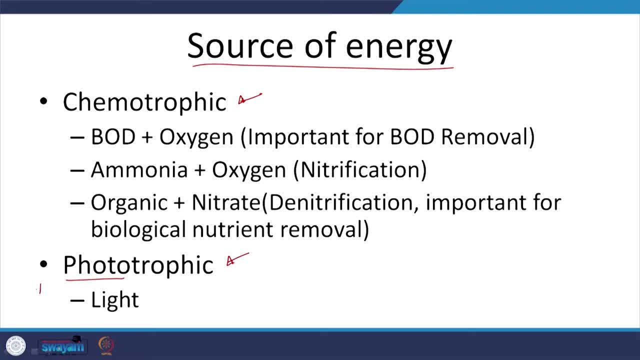 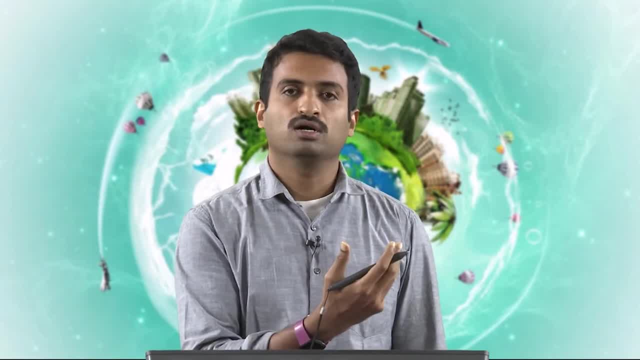 is light. source of energy is light, but we are not concerned with that. though if what we say algae or such- typically what we say are- depend upon what we say light or photo sensors, we are not really concerned with that because that is of no use to us. 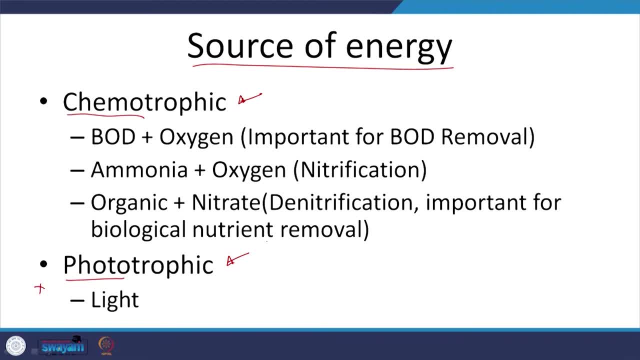 So here, chemotrophs- chemotrophic as in the sources of energy, or chemical or chemical sources of energy. This is what these are the microorganisms we want to make use of. What is it that we do? For example, BOD or the waste or our organic content, or our waste or the organic content. 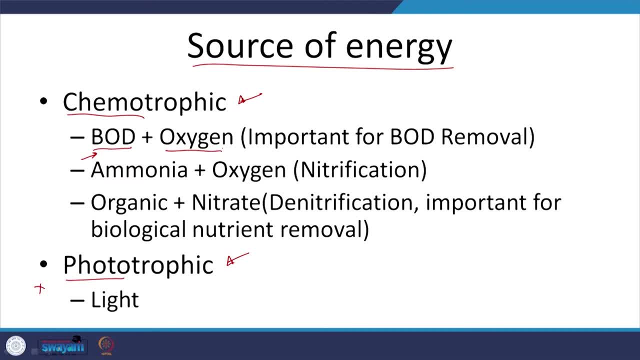 which is measured by BOD, can be removed in the presence of oxygen or oxidized in the presence of oxygen. So thus we are going to use for our waste removal. Another aspect is we also give out ammonia, and this is also, as you can see, a reduced form of nitrogen, and we have oxygen as an electron. 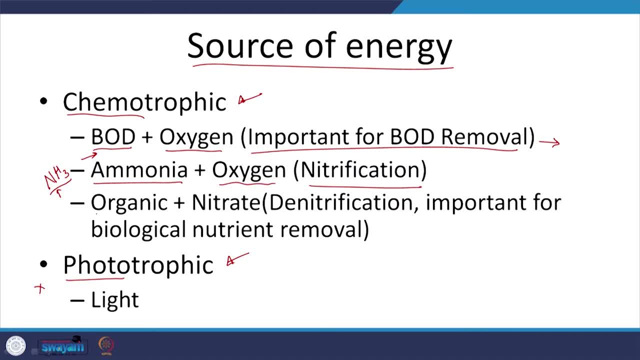 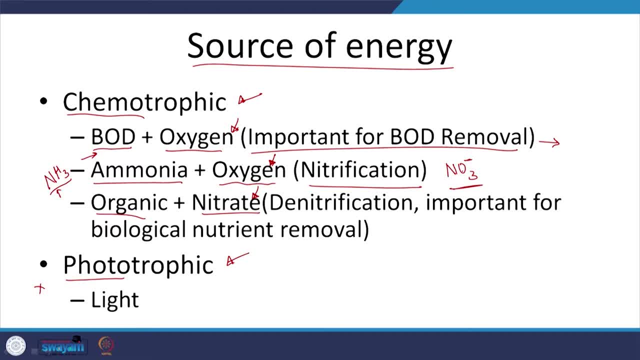 it in water, because it leads to adverse effects in humans and certainly in the aquatic systems too. So once you convert this NH3 into NO3, you want to remove this from water. How do you do You? by promoting formation of nitrate, nitrogen gas, pardon me, and that is called denitrification. 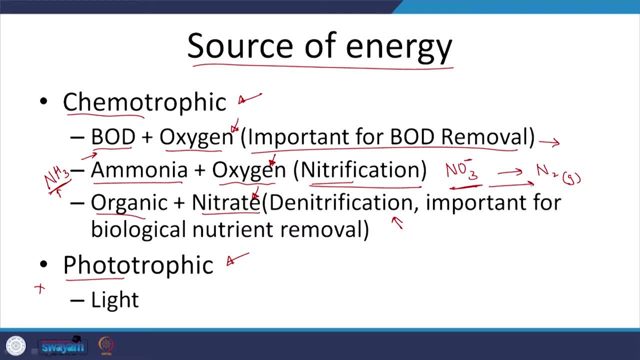 First one is nitrification, and then is denitrification, as in we are changing this from the aqueous phase, water, to the gaseous phase. Thus nitrogen is leaving our system. So sources of energy, in this context, one aspect to understand, or another aspect. 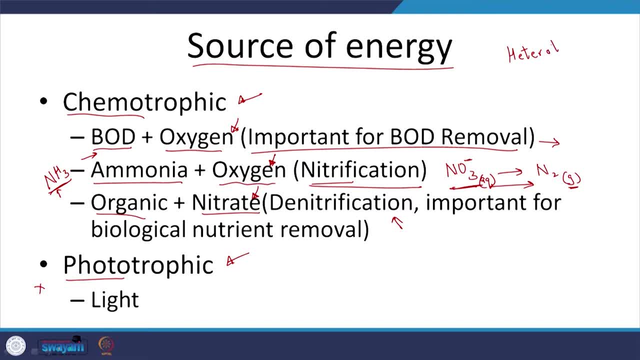 is that we have heterotrophs- heterotrophs- hopefully my spelling is right- and autotrophs. So one depends upon organic compounds or organic sources of carbon and the other on inorganic source of carbon, namely carbon dioxide. So obviously, as you can see, this is what do we say, even 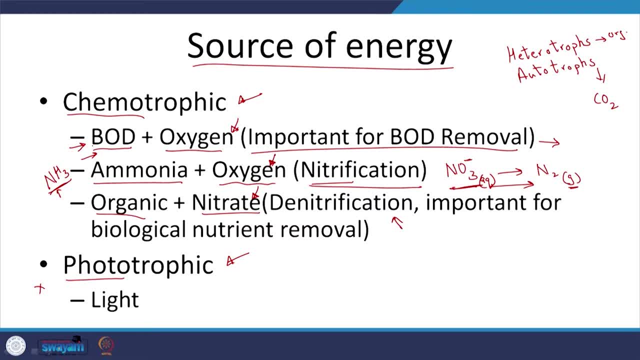 with respect to heterotrophs are done by heterotrophs, let us see right. And then nitrification, typically by what is it? autotroph, chemoautotroph? Let us see again. you need to, no need to mug up anything but for the serious listener or such. I am just 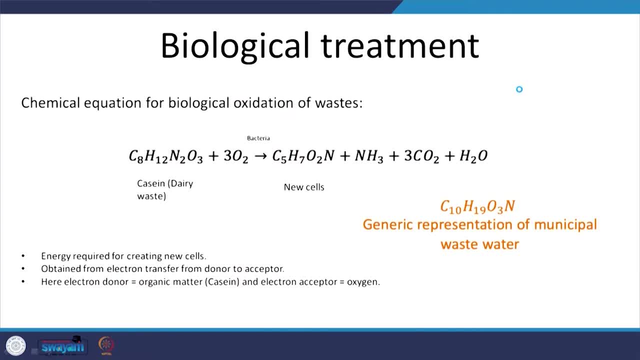 providing some information. So, biological treatment, let us just understand what typically happens. So, casein, a kind of a protein, I believe. right, we have it in the dairy waste. let us see. And here, what are we trying to do? We are trying to oxidize it, but again, as I said, 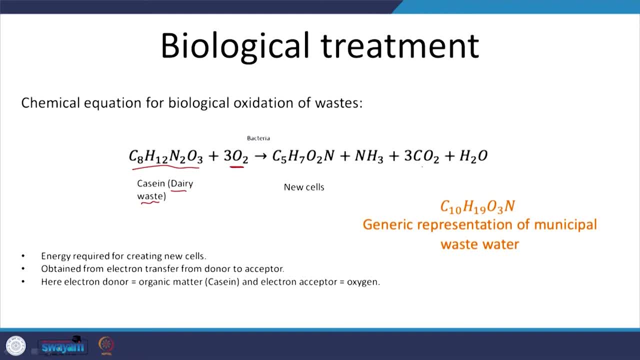 the kinetics, as in the rate at which this reaction goes through, is probably not good enough for practical oxidation by just oxygen. So what are we going to do? We are going to introduce bacteria which release enzymes. they release enzymes which act as catalysts, as in they fasten or improve the 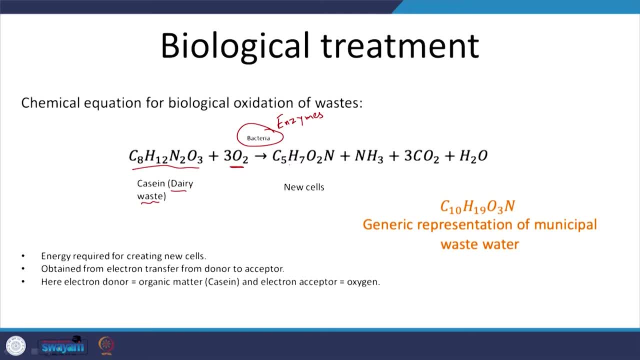 kinetics of the reaction. So here there are two aspects. One aspect is new cells, as in reproduction, as in new microorganisms, are formed. So cell synthesis, and then, while transforming it into other, what do we say? byproducts, they gain energy. So then again they need the energy, I guess. So. 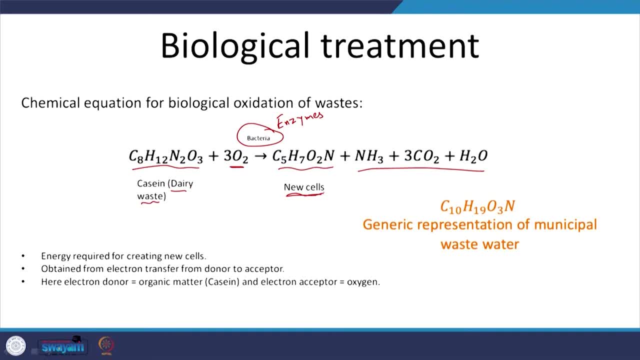 two aspects, one for energy and one for cell synthesis, And obviously, as you see, these compounds are relatively stable. carbon dioxide leaves the atmosphere. we have byproduct of water, NH3, which, if required, we will degrade further, So energy is required for creating new cells. 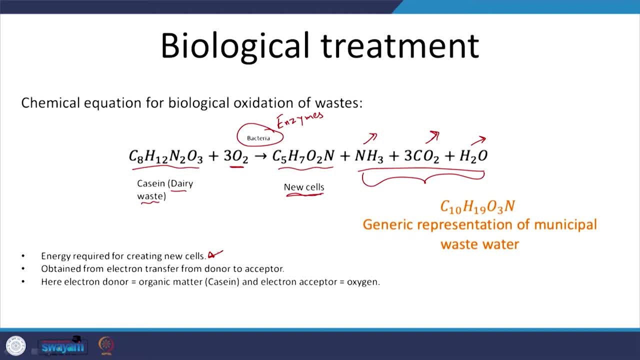 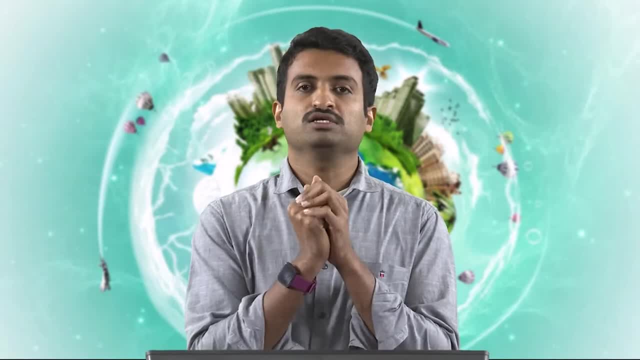 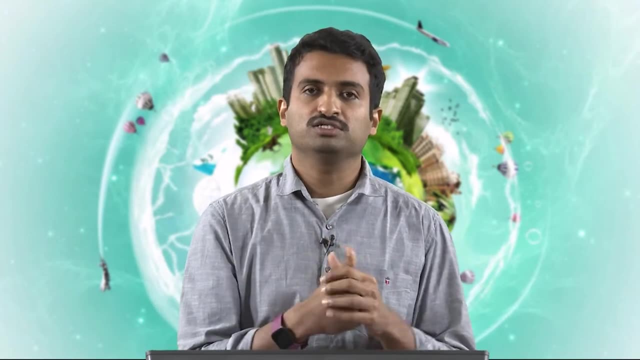 And how do we get that? For example, we have redox reactions, explosions, explosives and such And how. there are two aspects there: sudden release of energy and also sudden change in volume. But how is this energy being released? Because there is an oxidizing agent, typically, and a compound that is relatively reduced, So you have a redox. 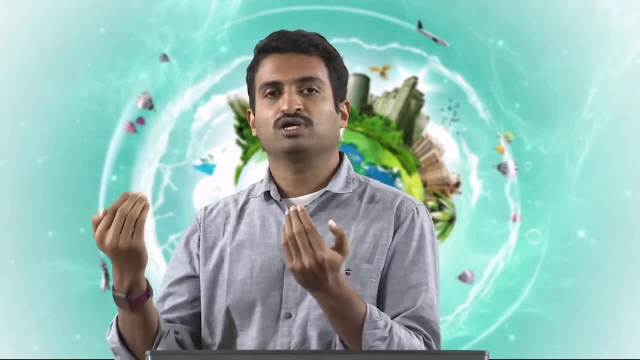 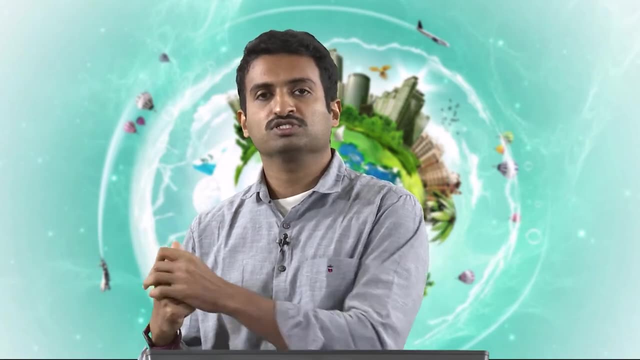 process, reduction and oxidation occurring, and then you are going to have transfer of electrons from the reduced compound to the relatively more oxidized compound, And thus you are going to have a redox process and plus release of energy. So that is the same principle here, Here, obviously. 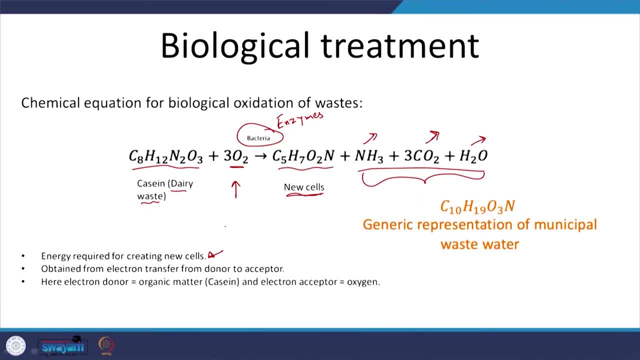 the oxygen is the electron acceptor or the oxidizing agent And the relatively more reduced form or the compound is this particular waste or R waste? You see, this carbon, that is typically the electron acceptor. Let us see Right, As you can see, it is bonded with H And here carbon is relatively oxidized. So that is. 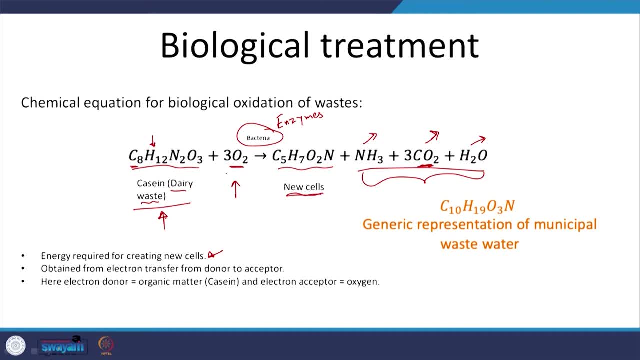 something to keep in mind. So let us move forward. So here we looked at electron acceptor. Let me just write that down. What is it that typically happens? A, which is relatively more oxidized, gains electrons and goes to its more reduced state. Here it is more oxidized and here it is. 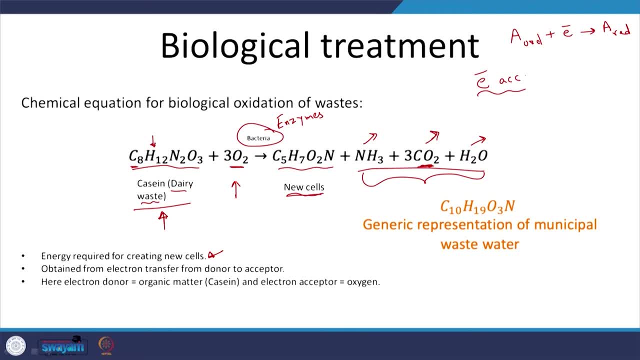 reduced, For example. here the example is O2.. O2 oxidation state is 0 and it is gaining electrons and going to H2O, where the oxidation state is minus 2.. Oxidized form of oxygen, reduced form, And similarly for the redox process to go through you, somebody has to, or some compound has to take this electron. 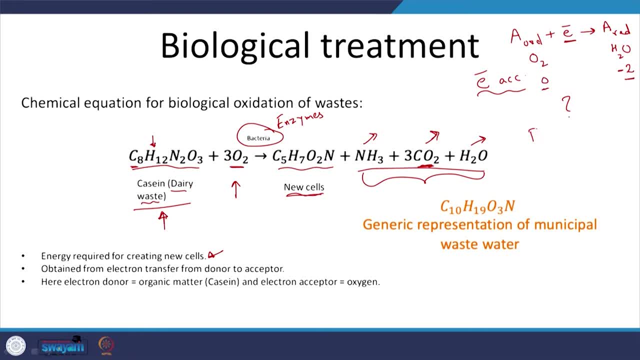 So who will take this electron? Let us see Right. So you will have. or who will give this electron? pardon, that was a minor error there. So here: for this oxidized compound to be reduced, somebody has to give the electrons, So you need an electron donor. 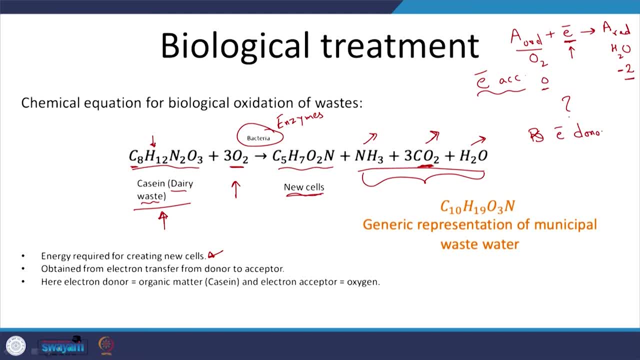 Let us see. Right, You need an electron donor. So who is the electron donor? as you can see, it is this waste or R compound. So the reduced, or B, let us see. B, which is reduced, will go to the more oxidized form and give out electrons. So this is the. What are these few? Let us see. 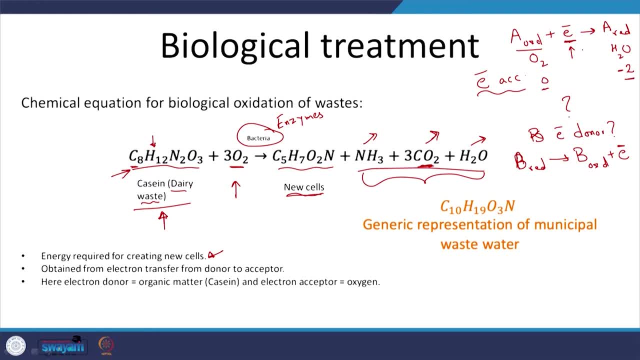 So this electron will be used by this particular half reaction there. So we have two half reactions. So here, what is the reduced form? it is the casein, I guess, and this is the reduced form. and what is the oxidized form? as you can see, it is carbon dioxide. 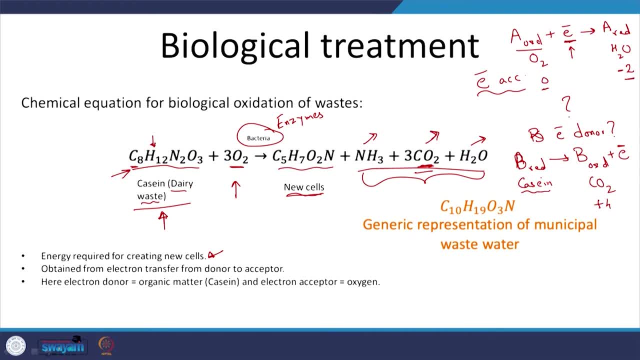 Oxidation state. here is what is it now, plus 4.. So you can look at what the oxidation state of carbon is in this particular compound. So this is the general aspect. So for wastewater, you know, for representation purposes, a general what do we say based on? 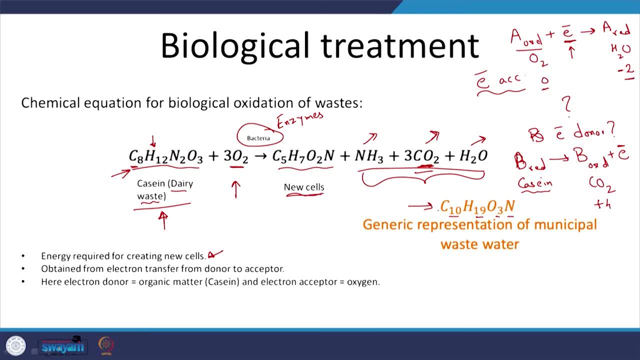 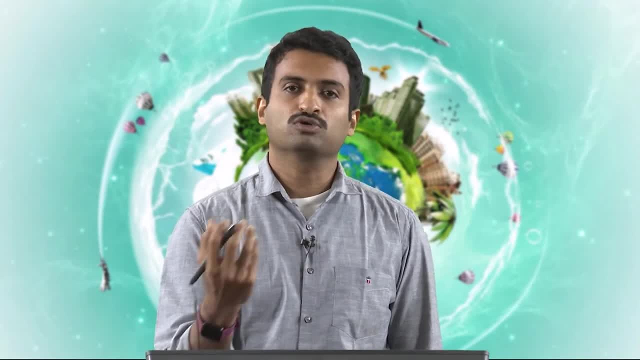 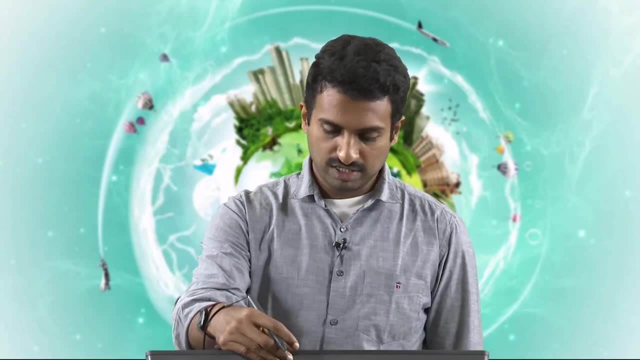 general ratio of carbon hydrogen, oxygen and nitrogen. this is the value, but again, there is no one particular. what do we say? value? not value compound or such that we can use as being representative of all the kinds of wastewater. that is something to keep in mind. 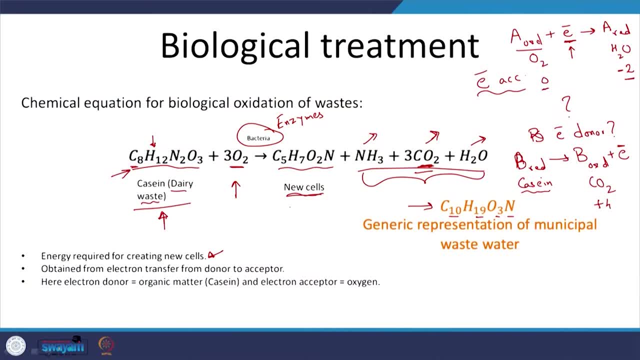 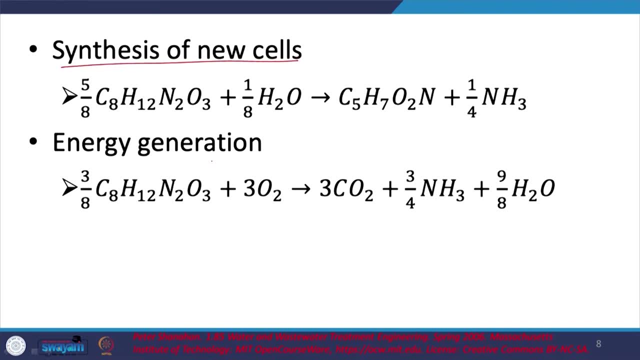 So from this redox process you can gain energy. but, as we mentioned, there were two aspects. let us see if we have that. So there are two aspects are One is synthesis of new cells. I mean the cells or such would not come out of thin air. 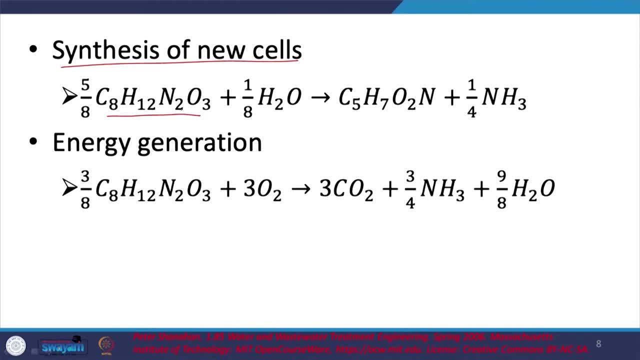 So you are going to have breakdown of this particular compound and have formation of cell synthesis. You can look at the stoichiometry, but we are not going to go into that detail. go into that detail, So: energy generation, different fraction. now, oxygen is the electron acceptor and then you 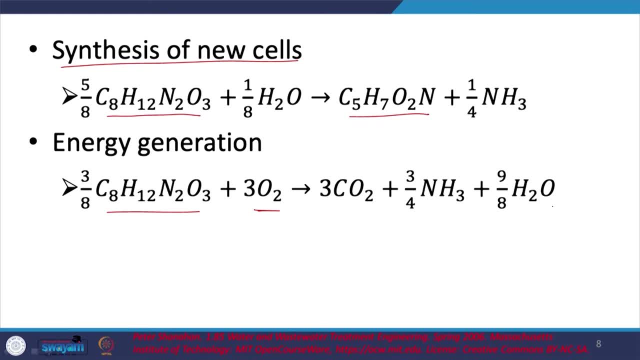 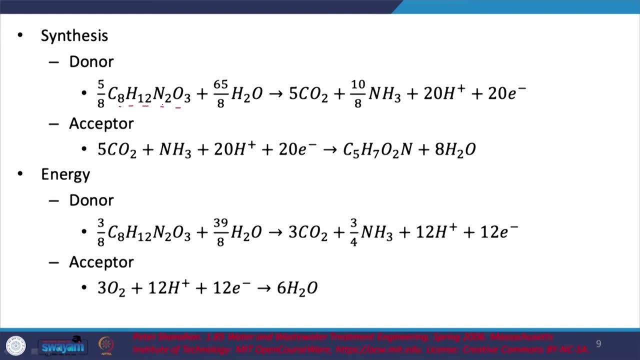 have the relevant byproducts. So two aspects out here. I broke down that equation into two aspects Here. for each reaction here that we have, we are going to have two half reactions. Let us look at that. So for cell synthesis, the donor here let us see the donor, electron donor. it is giving. 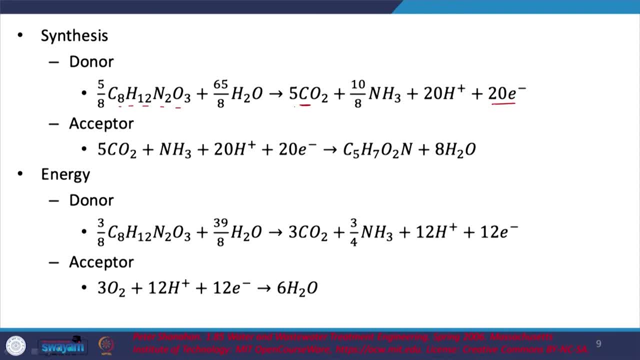 out these electrons. In that process carbon is being oxidized. So you can check the oxidized state of nitrogen and such. but primary focus here is carbon. Carbon here is relatively more reduced And by giving out electrons it is going to a more oxidation. I mean oxidized form. 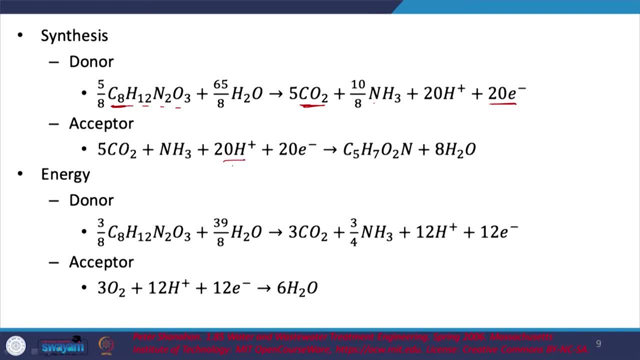 And these electrons. who is accepting that? So again, so I guess we have some error out here. So it is 20 H plus. I thought it was an error. So that is 20 H plus. these electrons are going to be used for cell synthesis. 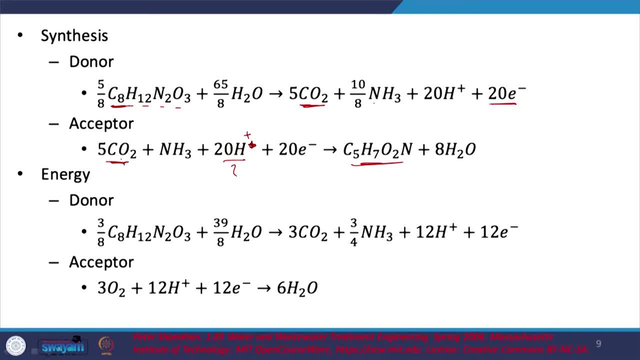 Carbon dioxide is again the electron acceptor. Let us see. Right So, because when we club the two half reactions Then we do not see these relevant aspects. But this role of electron acceptor is more clear when we look at energy. let us see: 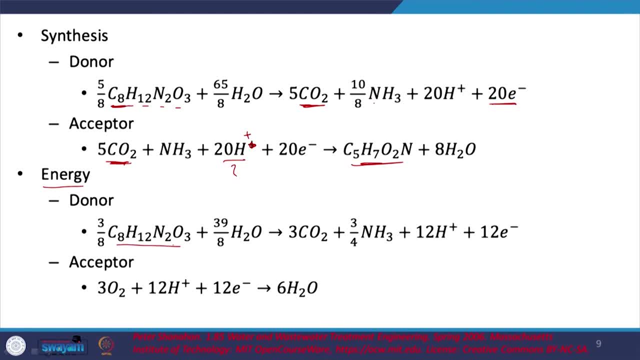 So what is the electron donor? It is still the relevant waste water or our waste, And we see electrons being given out and the more oxidized form. What is the electron acceptor? It was oxygen, and that is what you see: Oxygen going from zero oxidation state to minus 2 out here by taking up these electrons. 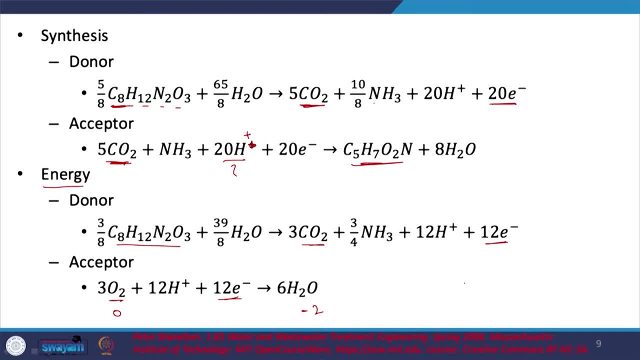 let us see, Right, So that is what we see out here In this process. We have these, which I guess is again used in this particular reaction. let us see, So there are different what we see: electron acceptors that you can use. to what do we say? 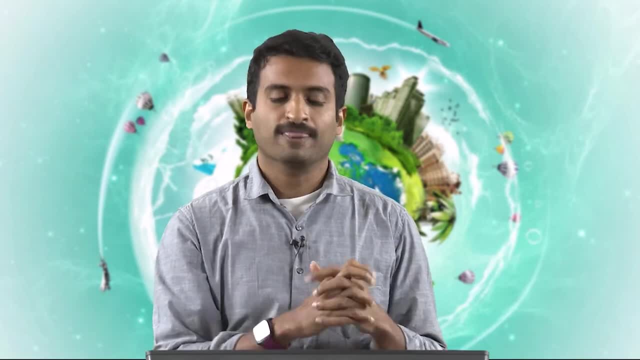 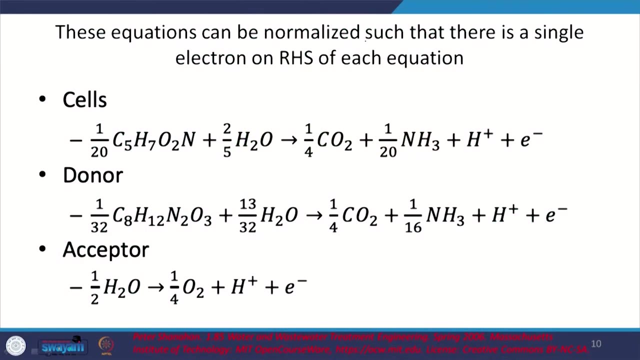 achieve different objectives. So let us just look at some of the different electron acceptors. Okay, So I guess I skipped one other aspect. So if I club these reactions such that there is one electron on the right hand side of each equation, So cells, you have this. 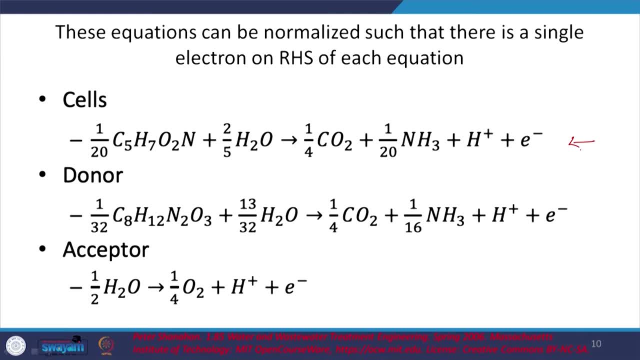 And the donor case. you have this For cells And for the donor And the thermal electron acceptor you can say is going to look something like this, But again, we do not need to go into this detail here. So, as I mentioned, we can look at different electron acceptors, typically the most what? 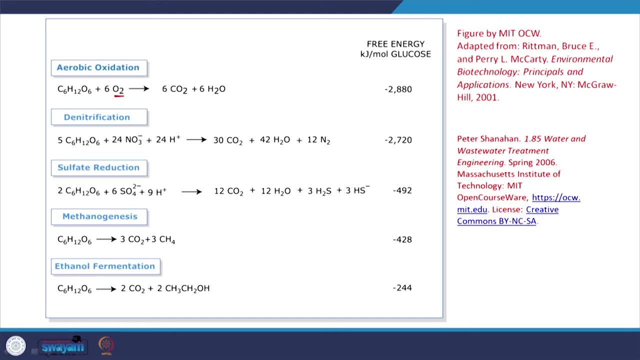 do we say, widely available electron acceptor is oxygen, as we see out here. So here we have glucose and glucose being oxidized to form carbon dioxide and water, And here we see 2880 kilojoules per mole of glucose. That is the energy that is released. 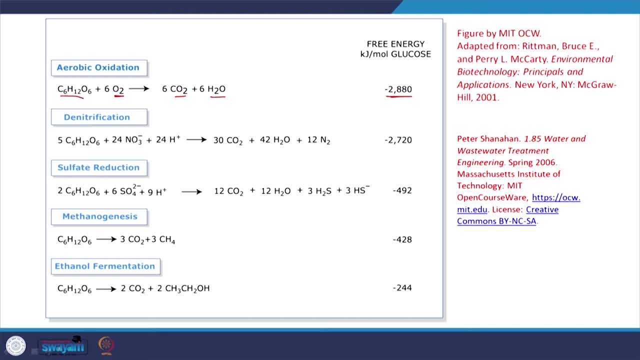 And if it is in denitrification, the electron acceptor is not oxygen But, as I mentioned, the electron acceptor is NO3 minus. And so what do we see here? We do see similar, but not as high- what do we say? amounts of energy, as in the case of 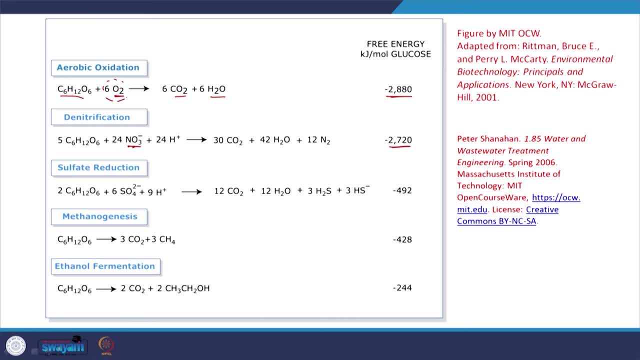 aerobic oxidation. Why do we say aerobic? obviously because oxygen is there. Here it is. there is oxygen, but it is not in the form of what do we say free oxygen? Okay, If I may say so, it is. the electron acceptor is NO3 minus. 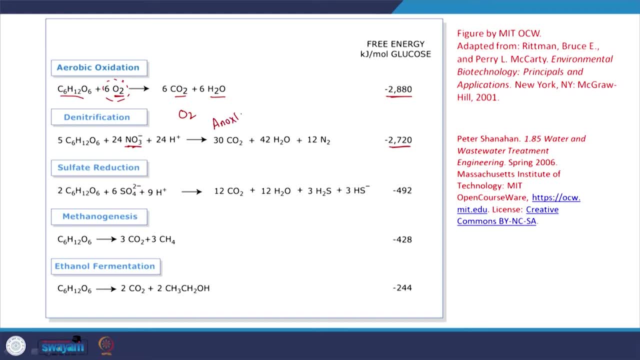 So these conditions we call as anoxic, right anoxic conditions, There is still an electron, what do we say? acceptor in the form of oxygen, if I may say so, not oxygen. Let me not make it more complicated here. we have oxygen and the electron acceptor, but 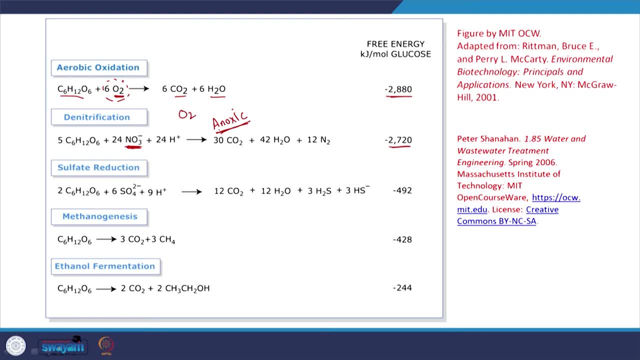 not oxygen we have. we call it the anoxic conditions. let us see right, And then you know you have different other. what do we say? electron acceptors, Sulfate- out here, right, And sulfate is reduced to hydrogen sulfide and less energy, as you can see. methanogenesis: 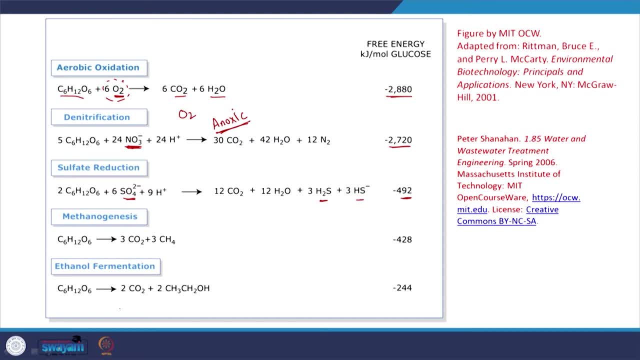 let us see right. and fermentation, where you do not have- what do we say, an external respiration mechanism here with respect to the cells. But as you can see, you know, as we look at different electron acceptors or fermentation and such, we see that the energy being released decreases. 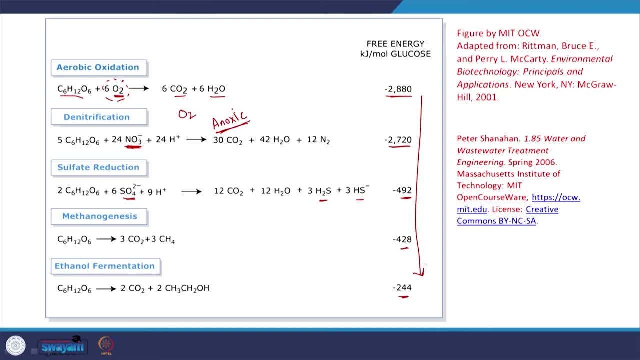 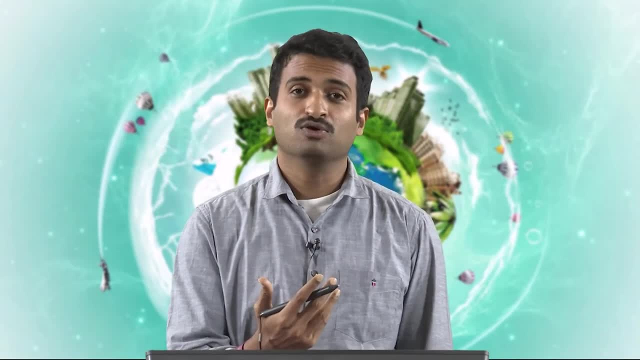 So microbes, again similar to us or human beings. So the students: they do not want to take my class because they need to go through a lot and need to submit a lot of- what do we say- heartbreaking homeworks. So they will take the path of least resistance. they will go to the relevant person who will 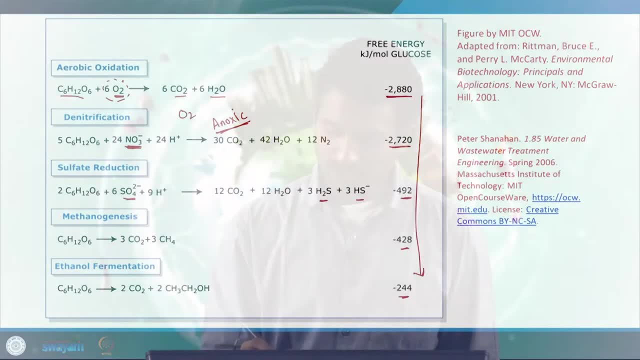 give easier grades with lesser work, right? So again, microbes too, they want more energy, right? So typically, I guess, looking at this analogy- let us say right Lehmann's analogy- we see that typically aerobic oxidation is preferred. Only when there is no oxygen Will this denitrification take place, right? 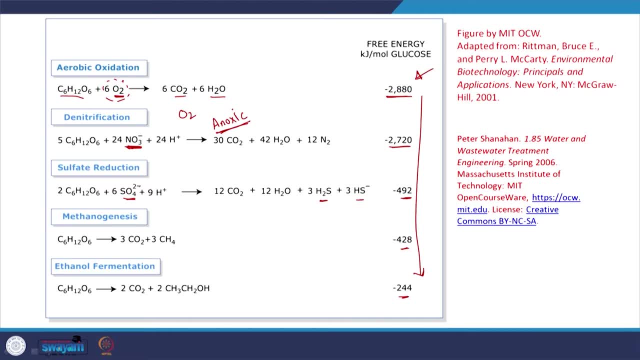 So that is something to keep in mind. And when there is no nitrate, only then if there is sulfate will this reaction go through again. different microbes are going to be prevalent at each. what do we say are going to carry out each of these reactions again? 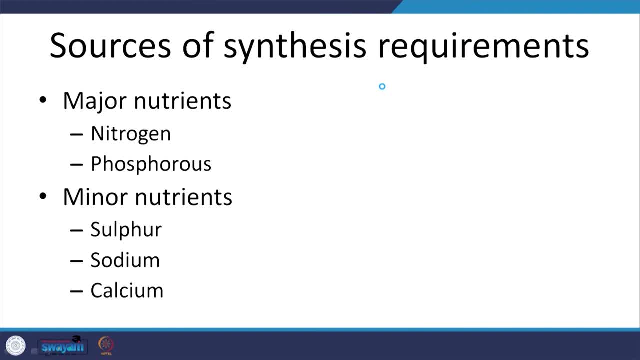 Why do they do that? because they want to get this energy. that is something to keep in mind. So what else do they require? One is energy, which we just looked at, and different electron acceptors lead to different amounts of energy. Okay, What is the requirement? 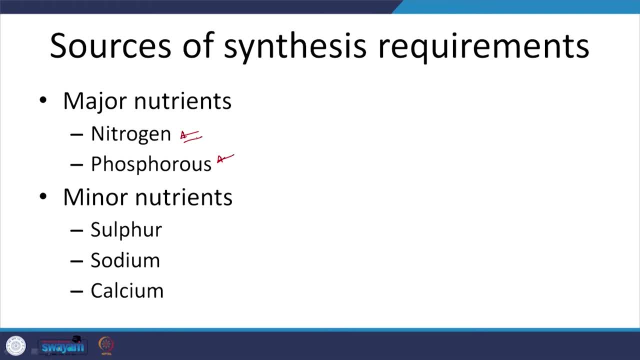 What do they need? similar to us, they need nitrogen and phosphorus. We typically take in nitrogen in the form of amino acids or proteins, let us see. And other nutrients are also required: sulfur, sodium, calcium and so on and so forth- But they are required at much lesser concentrations compared to nitrogen and phosphorus. right. 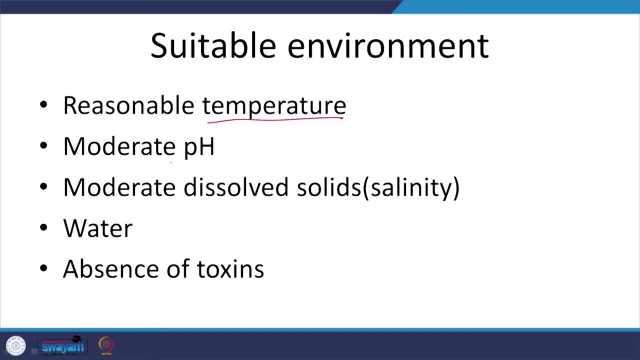 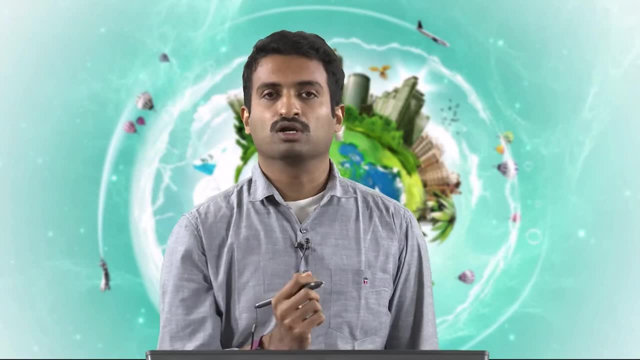 And suitable environment. similar to us, they want reasonable temperature, moderate pH, right. They do not like too much salinity. Total dissolved salts should not be too high. Obviously water and again, if you have toxic compounds coming in along with the wastewater, they are going to obviously affect the growth of your microbes. 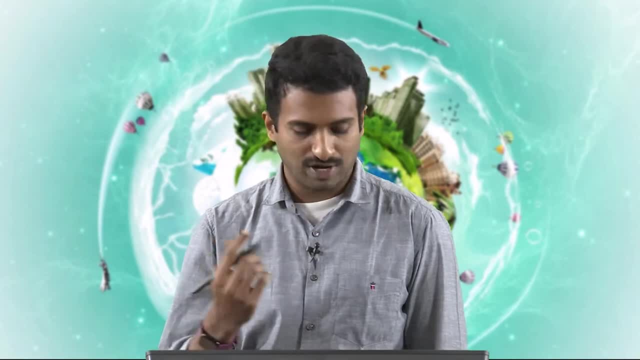 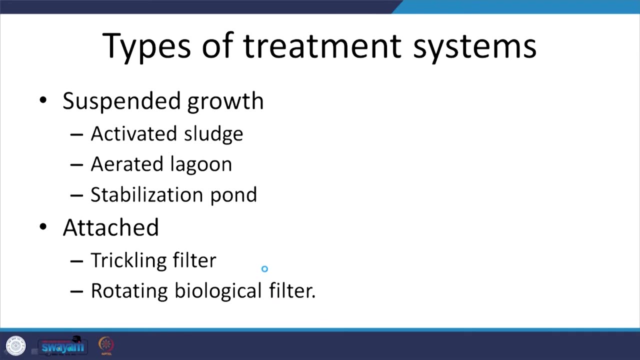 They can do the job, but maybe not as efficiently and they do not thrive as much, So they do not like a lot of toxins to be present in the relevant environment. So types of treatment systems: one, as we mentioned quite often, was activated sludge. we will look. 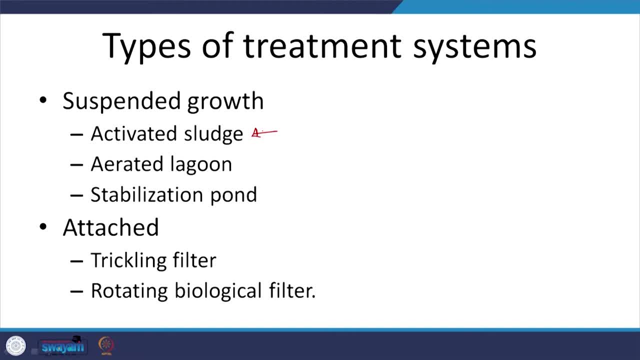 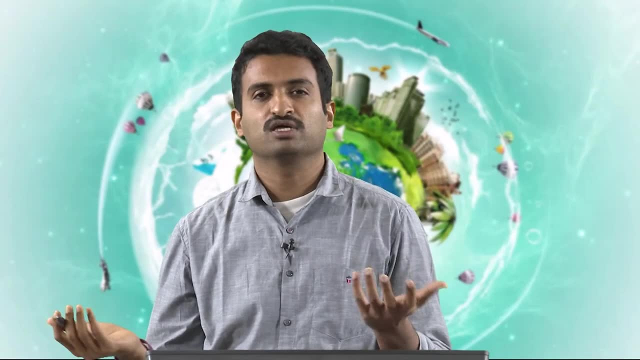 at a video two sessions down the line And earlier, when you know the concentration and also the flow rate were relatively less and land was available. people used to look at aerated lagoons and stabilization points, But we will not look at that now. people are facing that out, at least in India. let us see. 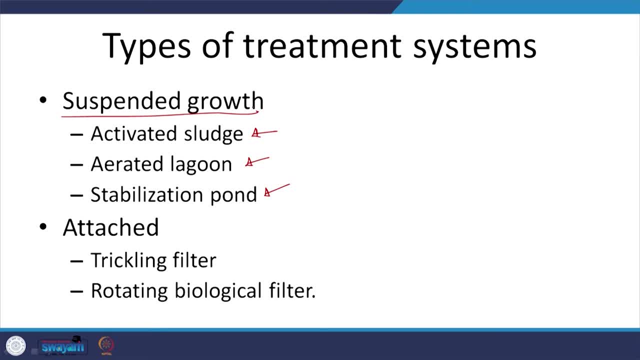 So the key difference between this kind of system and this system is that here we have suspended as and if this is my tank and this is the water, So the microbes are suspended, right? Okay, So here they are attached, but attached on to what some media, for example, I can provide. 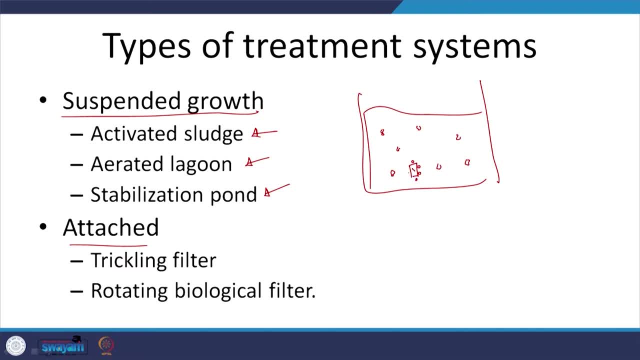 a media right upon which the microbes can grow right. So attached growth, let us see right suspended growth and attached growth. more often than not, people look at- have been looking at- activated sludge process, which is suspended growth of microbes, But sometimes people also look at attached and suspended growth to increase the efficiency. 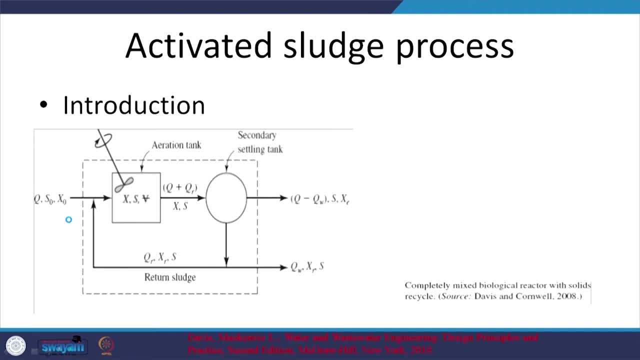 let us see. right, that is something to keep in mind. Okay, Activated sludge process again. why do we call that activated sludge? let us understand that. So I do have a relevant schematic here. we will come back to that. my wastewater is coming. 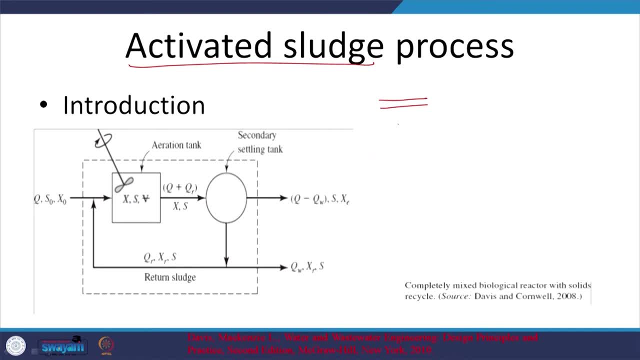 in. this is after the primary sedimentation. what does it have? it has a lot of organic content, which I am going to call substrate, which is my waste, and the. what is it? the food for the relevant microbes, but the concentration of the microbes in this relevant sewage, or 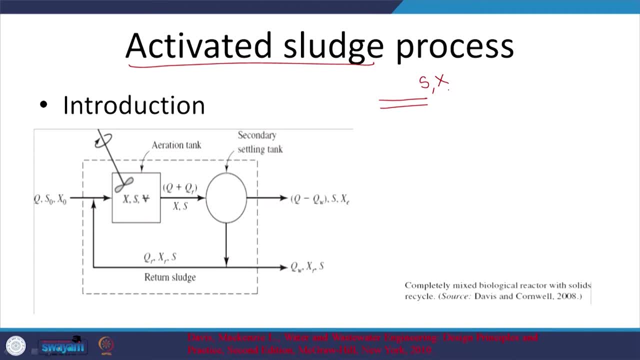 wastewater, Which I am going to represent by X, is going to be less right. there are going to be some, but not enough for what we say. fast degradation and also the kind of microbes that are present might not lead to what we say, the degradation of the kind that we are looking for. 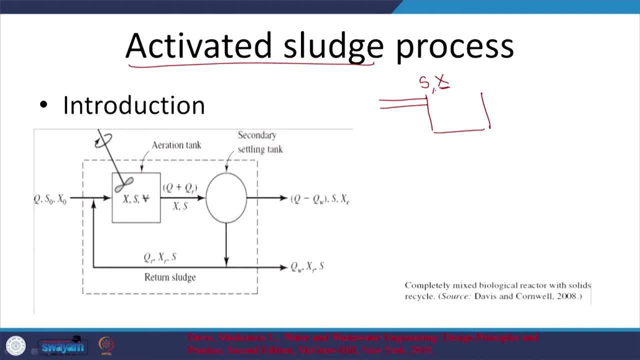 So what am I trying to do, or what do I want to do? I do not just want this X, I need a X that is remarkably high. So this is X naught and S naught. I need a concentration of X or the microbes in my tank. 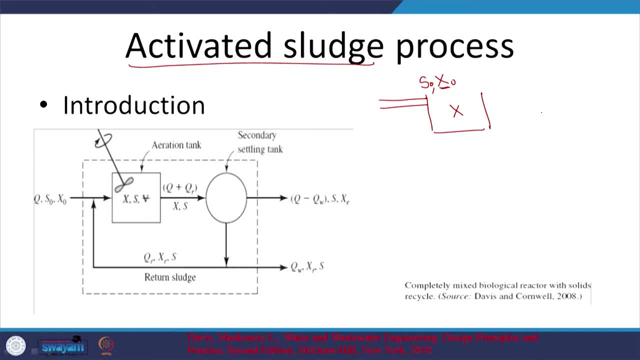 to be very high. So how can I achieve that? let us say so, I need a source of microbes, right? so I need a source of microbes. okay, let us see where this will come from. So, in this tank, what else do we need to provide? I am going to provide mixing and I am going 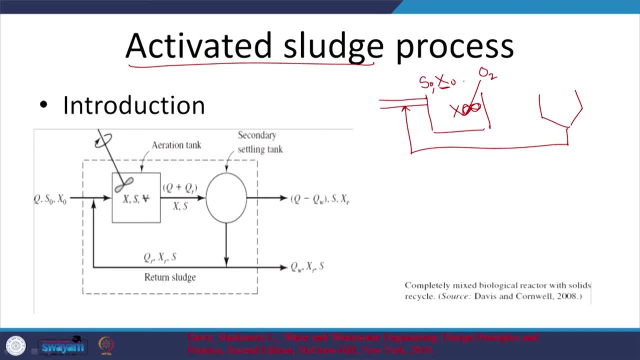 to provide oxygen. So here I am going to provide conditions such that the microbes thrive and the concentration is high. Once they we stop aeration, we send that to what is called a secondary clarifier or secondary sedimentation tank. What happens is, if we maintain the right condition, 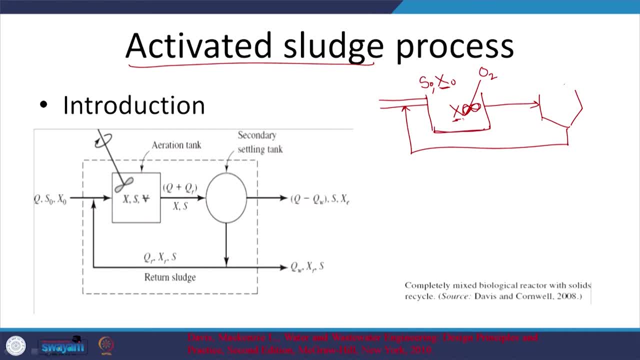 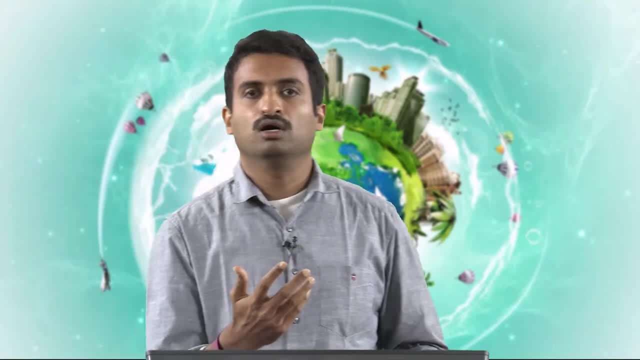 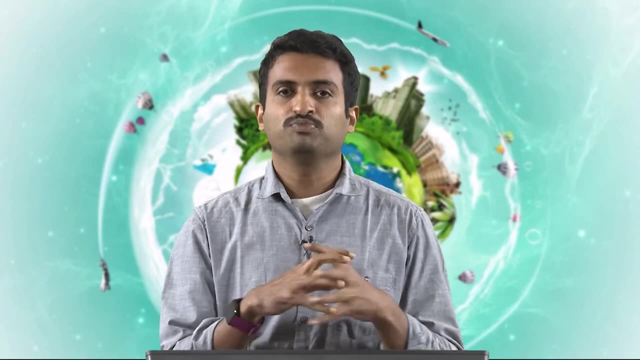 Once the kind of bacteria that form here include, or what we call flock forming bacteria, with some filamentous bacteria. So we looked at this figure, I think in what do we say? the last session, where you we looked at the microscopic pictures and we saw the flocks being formed along a filamentous backbone. 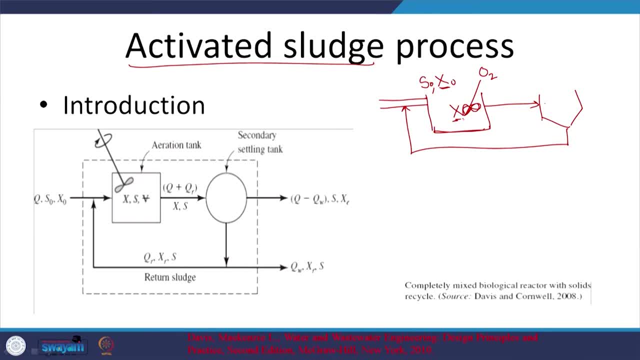 So these particular flocks or kinds of microbes, they are going to settle down. they are going to settle down And they are going to settle down at the bottom. So typically you can waste it or you can recycle that or for recycle such that when it comes, 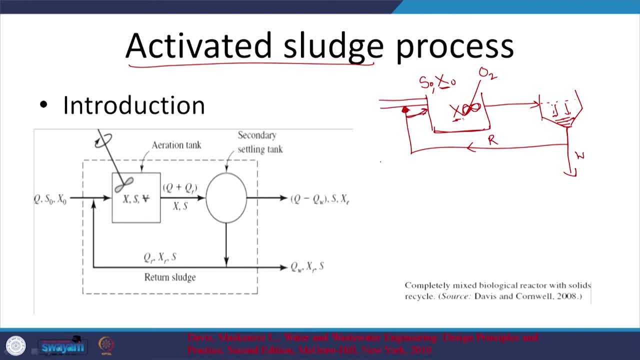 into. okay, I should not draw it here, maybe I should draw it right here. I can recycle it such that the concentration of the microorganisms in this tank, where the actual reaction and degradation takes place, is pretty high. So that is why we call it activated sludge, as in this sludge which has the microbes activated. 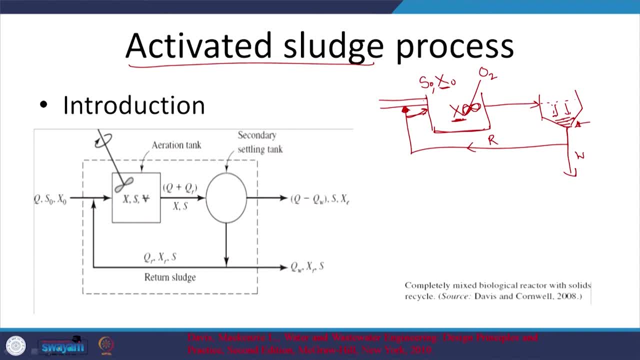 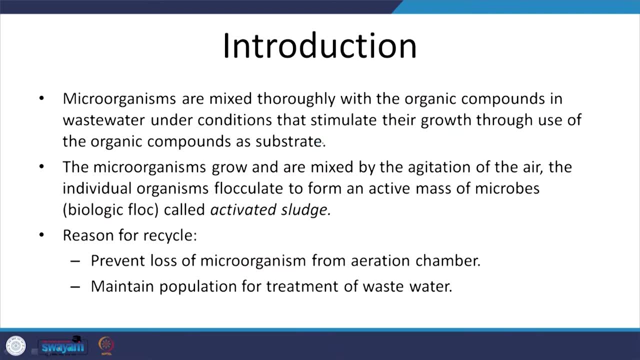 sludge is reused Right Activated sludge process. again, that is what we have. that is the relevant schematic out here. Let us move on. So I believe we already looked at this. So why recycle loss of microorganisms? right, you cannot keep bringing them and you want. 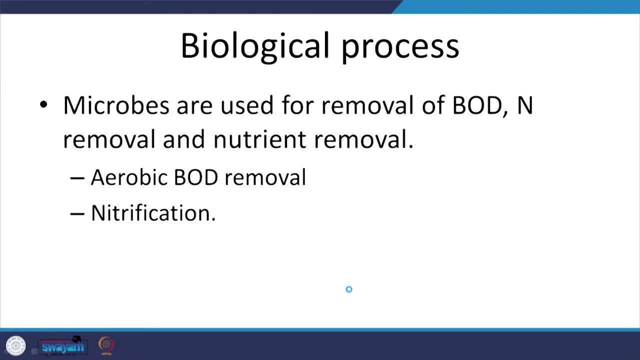 to increase the concentration. let us see. So we will skip this. And what are we trying to use it? obviously, depending on the design. you can decrease the organic content, which we are measuring by BOD. if the ammonia content is high, you can design it such that nitrification first. 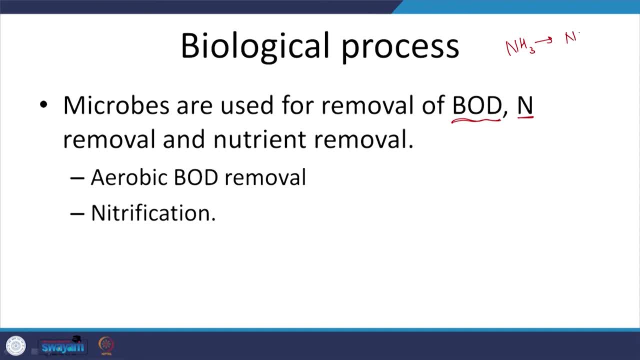 As in NH3, goes to NO3- and then, with denitrification, this is aqueous phase, and now nitrogen, which is in the gaseous phase, will be formed. this is nitrification, then denitrification, because we are forming nitrogen gas which will leave the aqueous phase or the water right. 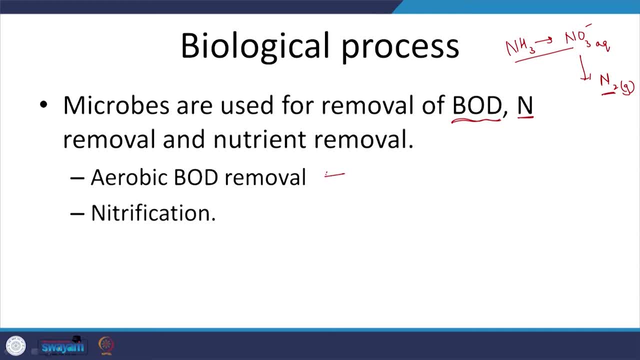 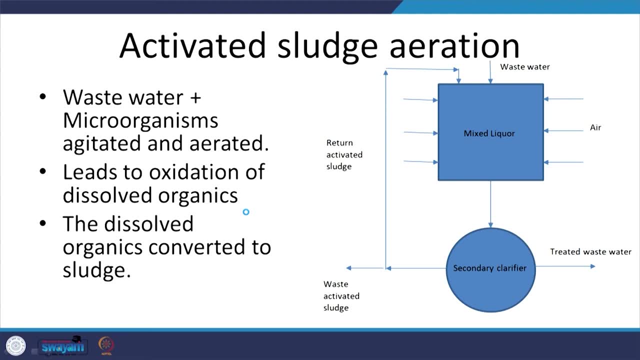 So we can look at the relevant aspects. So aerobic BOD removal, nitrification and such, we can achieve that. So activated sludge aeration- I guess We have a picture out here. we will, or we already looked at this in detail. but again, the primary 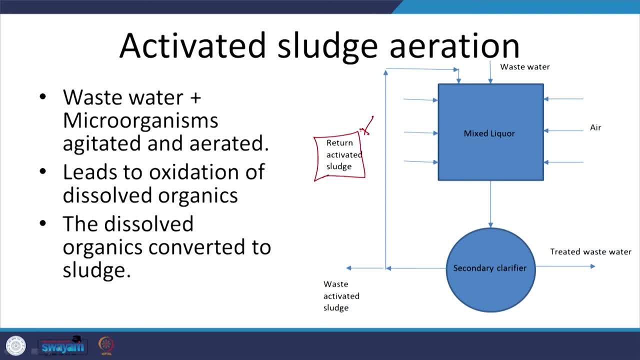 aspect is this: return activated sludge. One aspect to note here is that in India, people do not maintain these. what do we say? clarifiers or, you know, maintain the right, recycle right. What does that lead to? that leads to very low concentration of the microbes in this. 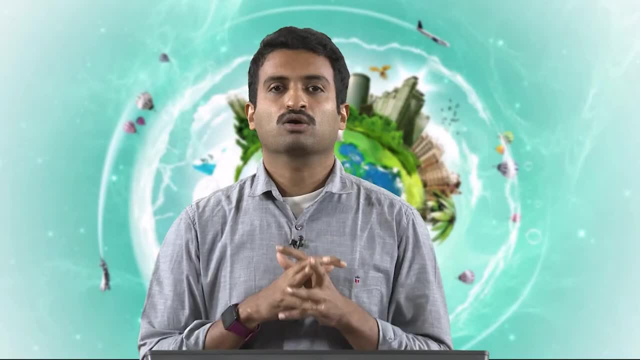 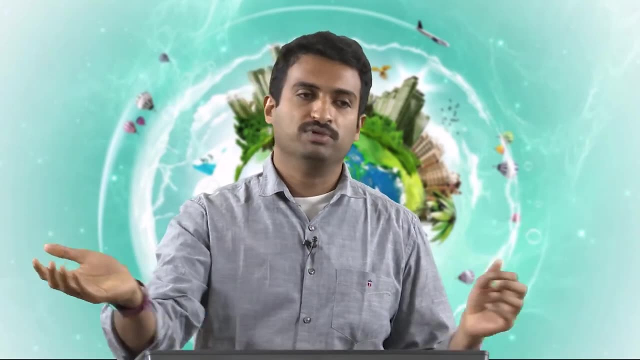 particular aeration tank. So what happens when you have less concentration of microbes? first the kinetics. right as a reason, let us say there is 10 kgs of Laddu and let us say 100 people faster consumption. let us see within maybe 10 minutes or so. 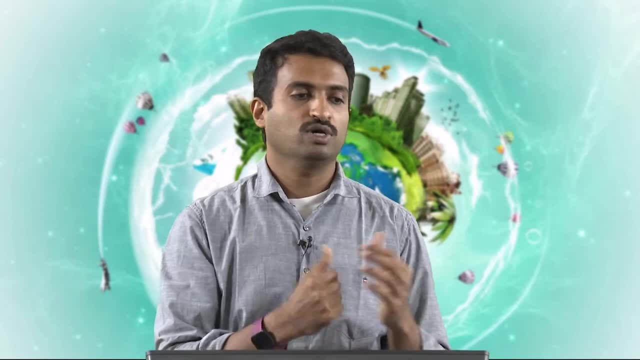 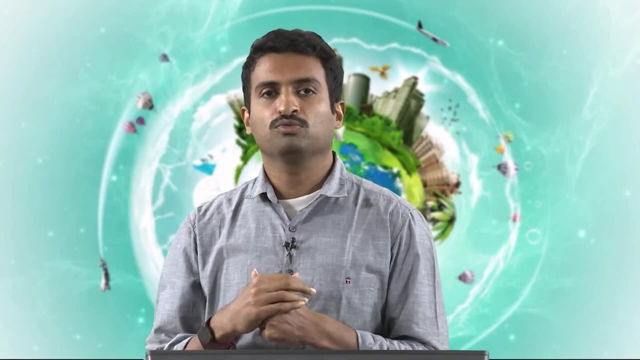 But if there is only one guy, obviously you know it is going to be an issue as in the time, or the kinetics are going to be pretty slow. So same case here: people do not maintain the right conditions for the microbial growth or do not maintain sufficient concentrations of the microbes. 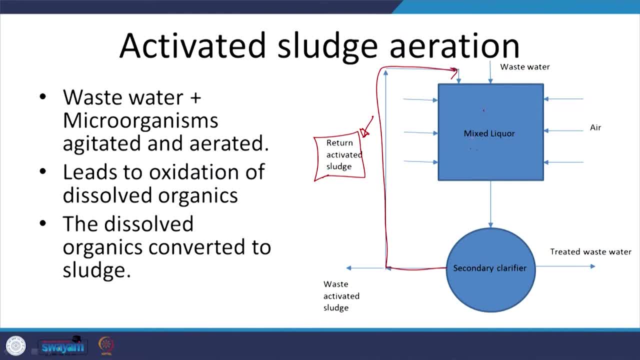 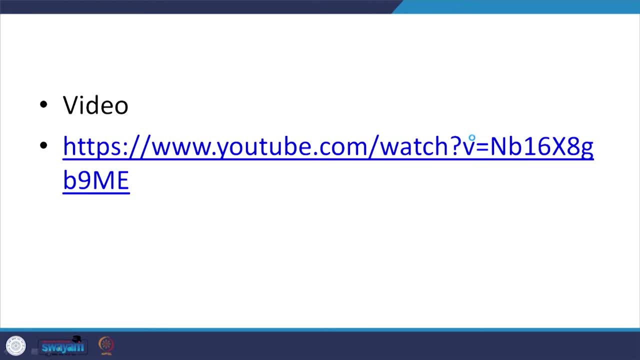 So that is why different treatment plants, either industrial or sewage treatment plants- and they are typically affected. Let us see, So, keep in mind, right? So I guess I have one video- you can look at this video, okay, which looks at different aspects, and I will play, or I will try to play another video that is out here. 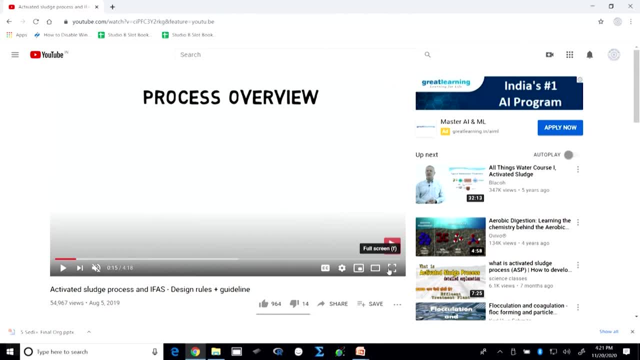 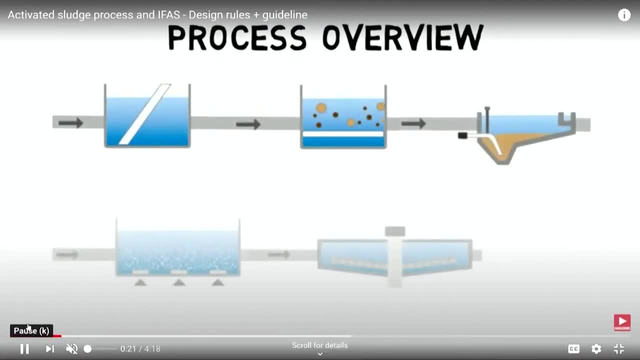 So you can look at the link and such and the reference. obviously we are just trying to look at the schematic. let us see right. So process, what do we have? we have the grid chamber right, or the screens, pardon me, cores, particles, rags and such. 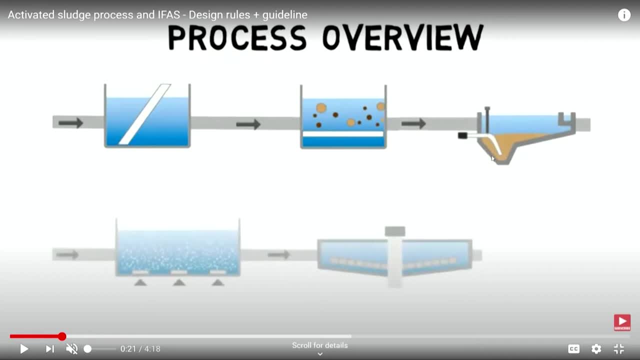 Then the primary sedimentation Basin right, and then you have the primary sedimentation basin out here, right Grid removal primary sedimentation basin and then we have mostly only the suspended matter, and here this I hope you can see the arrow- We have the biological process. where air is provided, microbes are coming into the picture. 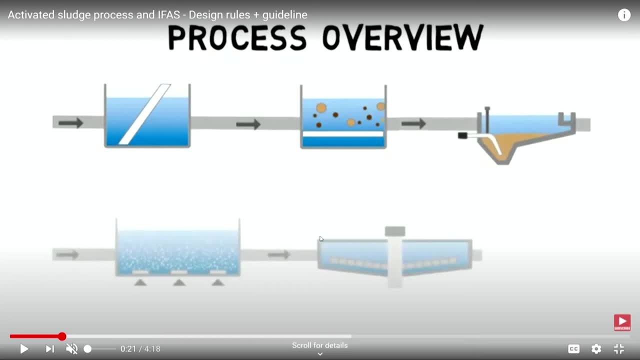 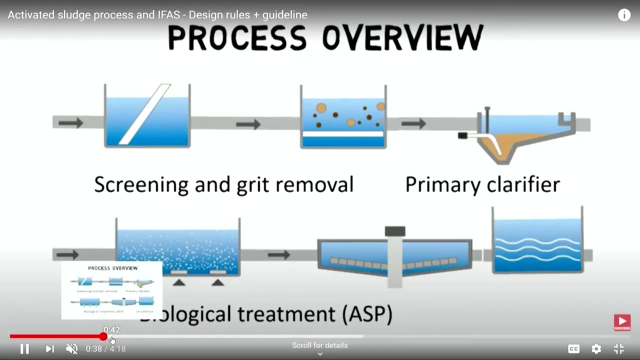 that is why the biological process and then the act, the secondary clarifier or secondary sedimentation tank, let us see, right, Let me just play this a bit further. Okay, Okay, Okay. So what we just mentioned out here and in the biological process, what do we see happening? 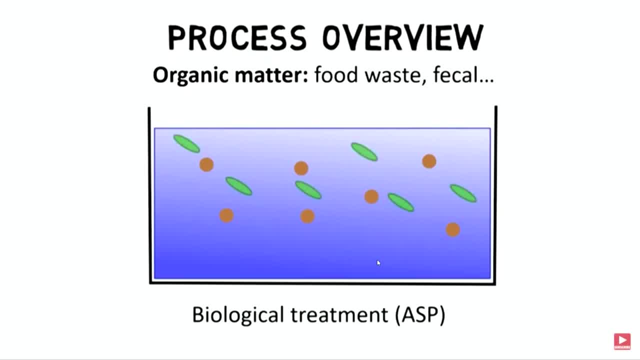 What do we have? We have our waste, fecal matter. We provide the relevant microbes, right. and then microbes are, what we say, going to degrade the organic matter to the relevant byproducts. let us say, right, But what do they need? They need an electron acceptor, which is oxygen. 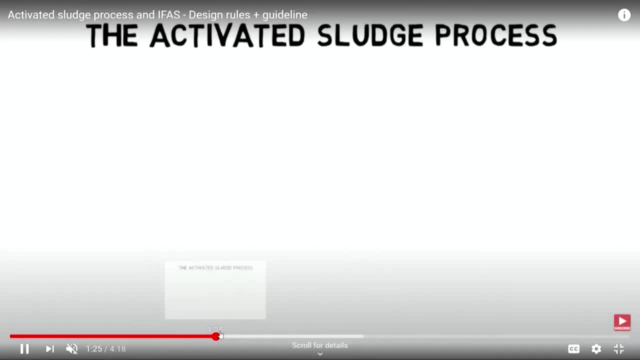 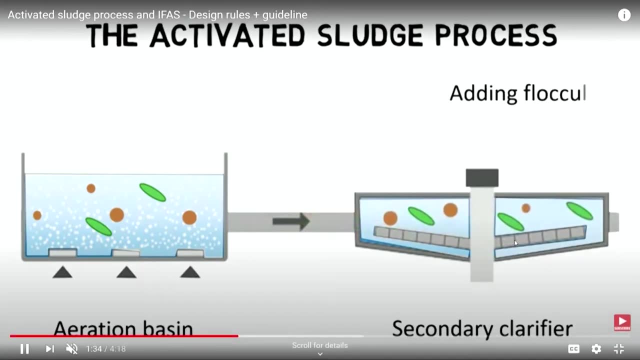 That is what we are providing here, right And then? so what do we have here? We have these microbes or flocs that come into picture here. Here this other, or the video maker, says: we add flocculants, but in wastewater treatment we rarely, if ever or never, add flocculants. 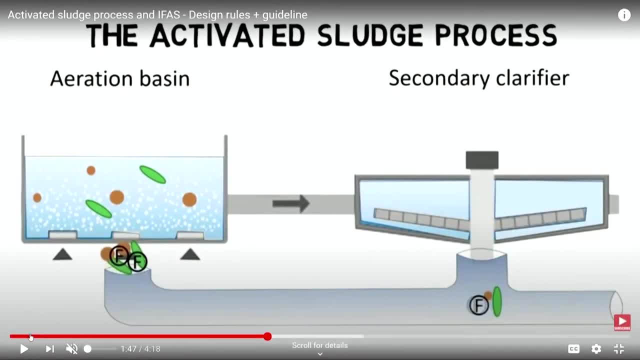 The kind of bacteria that are be going to be formed if we maintain the conditions to be good. They are going to see to it that this particular sludge settles down And some will go to waste And some is recycled back So that the concentration of the microbes in your relevant aeration tank is high enough. 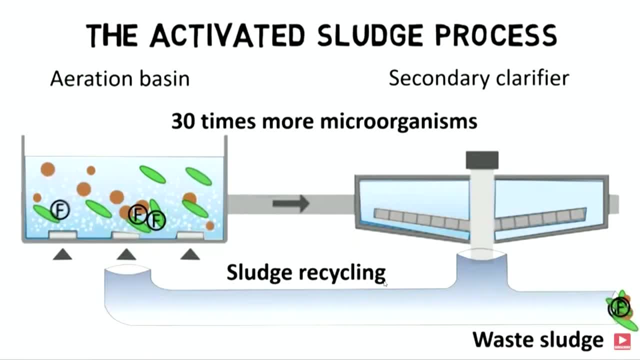 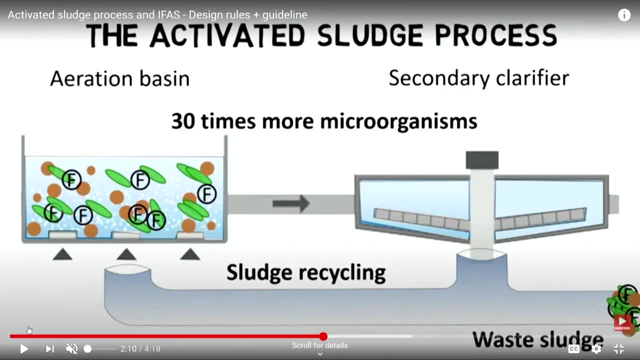 let us say right, So that is why we call it as activated sludge. The sludge which is activated is recycled and used out here. let us say right, So that is enough for now. but you can look at the other video, which is not a schematic. 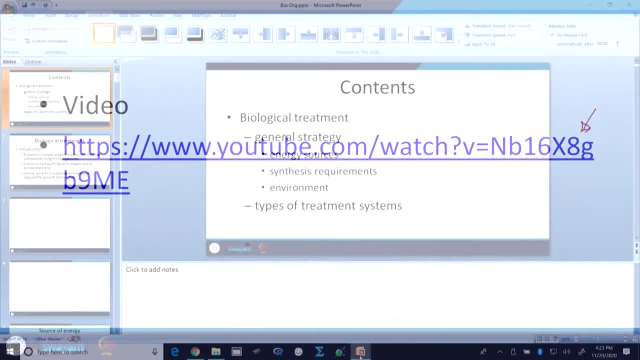 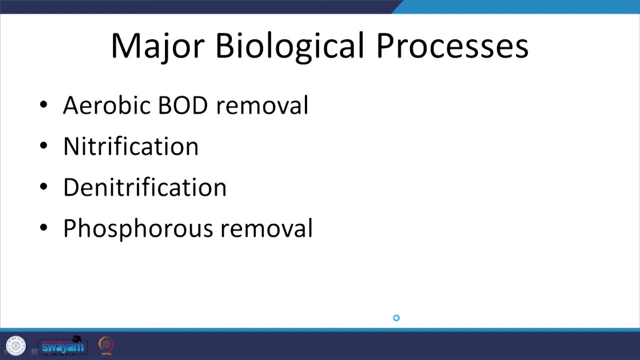 but from relevant treatment plant. let us say right, So let us move on. So what are some of the major biological process that we try to use? Okay, So, as we looked at in the class or sessions beforehand, we want to look at those compounds. 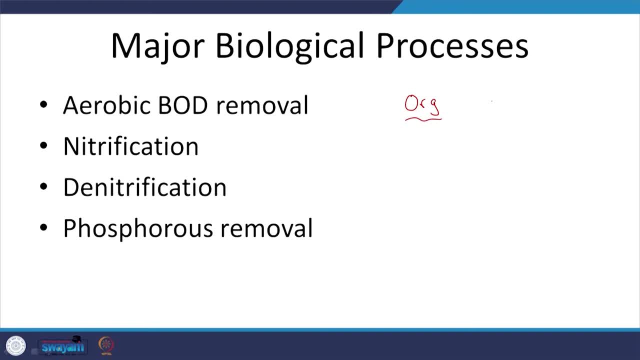 which have or exert an oxygen demand, or the organic compounds which exert an oxygen demand right. So this oxygen demand we were measuring by BOD. So we want to remove the BOD and also we mentioned, you know, algal growth and such. So we want to remove the nutrients depending upon the concentration. 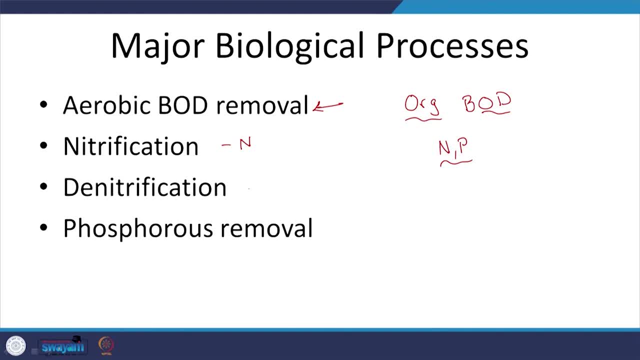 So we remove nitrogen, Okay, So by nitrification and then denitrification, and then we also look at phosphorus removal. Let us just briefly look at the relevant aspects out here. So nitrification, I guess we already looked at aerobic BOD removal in considerable detail. 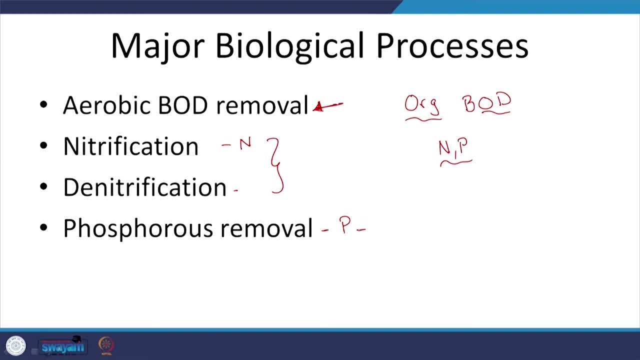 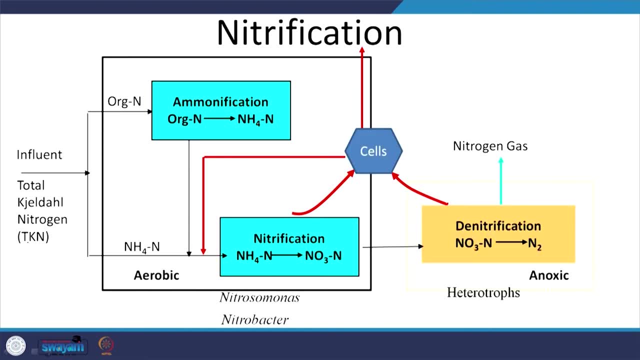 Let us just look at nitrification and denitrification briefly, and then phosphorus removal. We will come back to this later, but again, we are just understanding the principle here. that is something to keep in mind. So TKN: right, we know what it is going to give us, right? 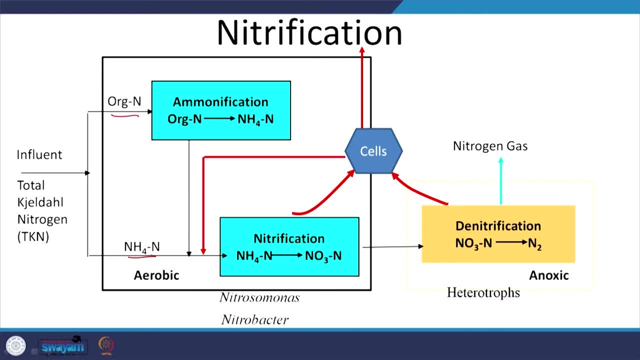 You have organic nitrogen and this NH4N- let us see NH4 or NH3N, and what is it that we are going to try to do by nitrification? this NH4N is going to what do we say, be transformed into or oxidized to nitrates NO3 minus. 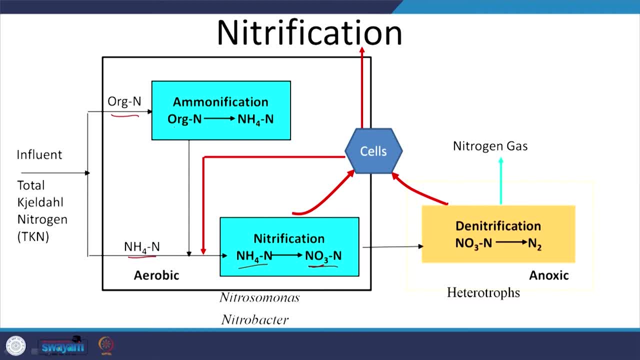 But again, this is simplistic diagram. we will look at that later and in during that time, obviously, the organic N will be degraded by microbes to NH4, right, and then that NH4 again to NO3 minus. But, as I mentioned, NO3 minus, Or the nitrate, is toxic to humans and you do not want it to be in the water. 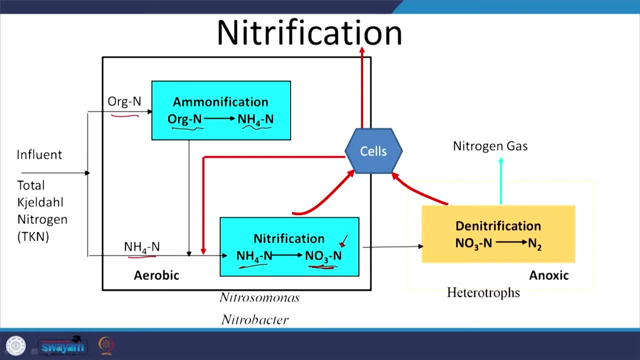 So you have to remove it, but again it is very soluble. What do you want to do? You want to see to it that it changes phase such that we can remove it. So that is where we have denitrification, as in nitrate NO3N, as in NO3 minus expressed. 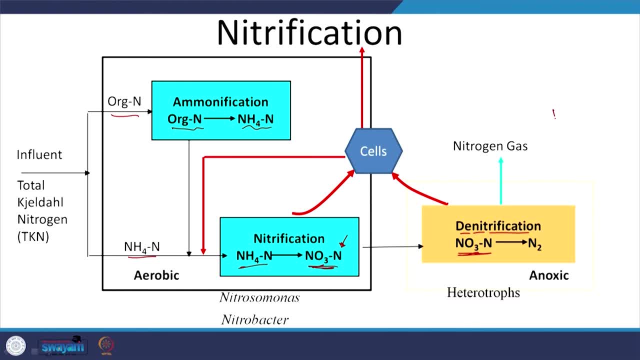 as N, So you do not need to really look at this. nitrate, which is NO3 minus, now is going to be reduced to nitrogen. But here the issue is: This is aqueous phase and this is gaseous phase, and then this nitrogen gas is going. 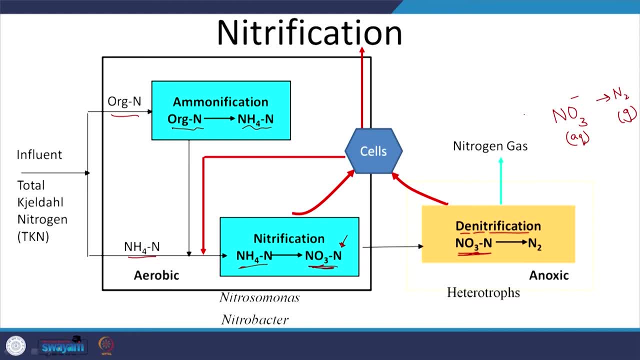 to leave the system. let us see. So that is something to keep in mind. But again, how is this reaction going to come about? Please note that this will not occur in the presence of oxygen. Why we looked at the relevant electron. I mean not electron transfer, energy generation- for 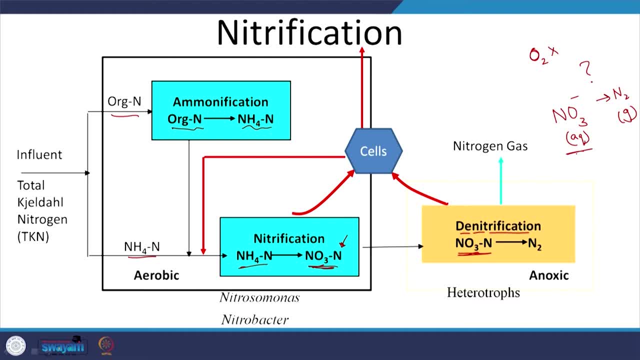 different electron acceptors and you would have seen that with this particular electron acceptor they do not gain a lot of energy. So If there is oxygen present, the different kinds of bacteria will thrive. let us see. So what do we need? We need a more reduced compound. let us see organic compound. and then what is it? nitrates. 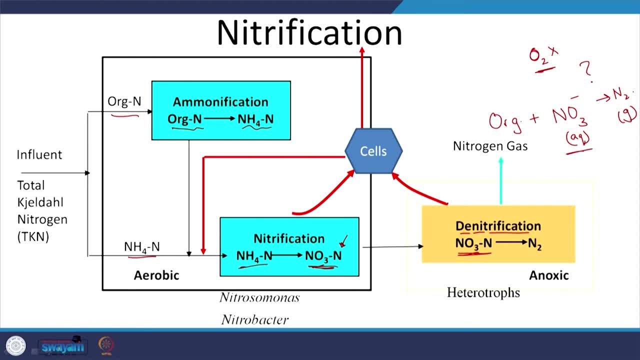 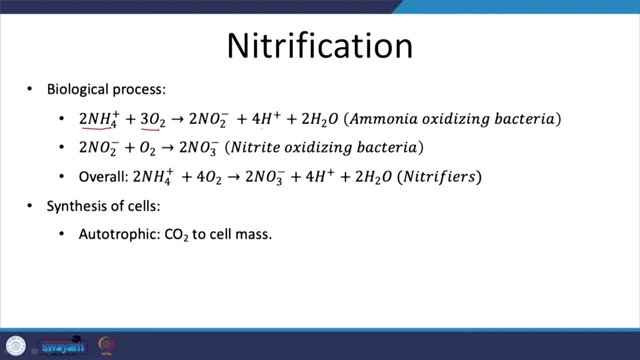 which are the electron acceptors, and that is what you will have. let us see. So let us look at the relevant reactions. So biological process, So ammonia oxidized by oxygen, but directly you would not have formation of nitrate first, you will have formation of nitrite and this is called, or you know the type of bacteria. 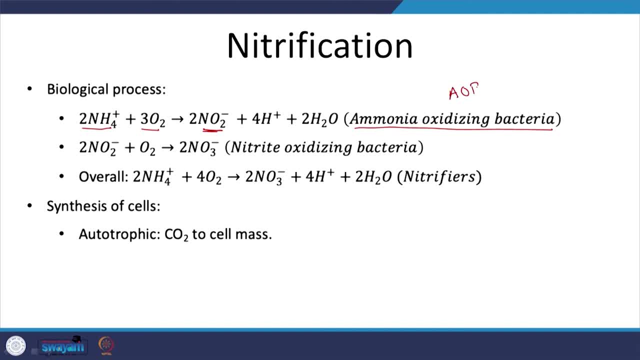 that do this, Or called ammonia oxidizing bacteria. let us see. So that is the relevant reaction. let us see. and then what happens to this nitrite? nitrite is further oxidized by oxygen to nitrate, by what we call nitrite oxidizing bacteria. 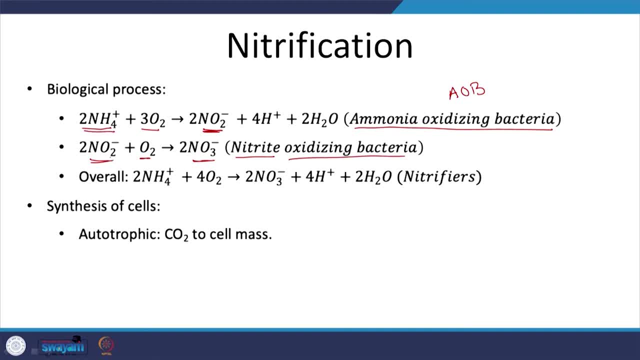 Here ammonia is being oxidized, and then here we have nitrite being oxidized. So, overall, though, if we cancel out nitrate, this is what it looks like, but please note that we have two kinds of- what do we say- reactions involved here. So 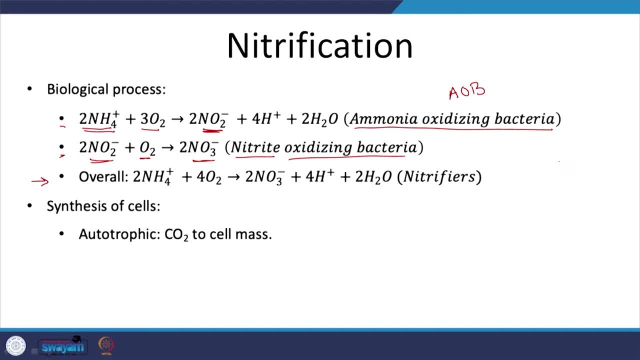 Here. One aspect to note that here is: we have no organic compound present here. no organic compound. So how do these bacteria grow, or not grow, cell synthesis? how does that occur? So they are autotrophs, not heterotrophs. that is why they use inorganic carbon to form their 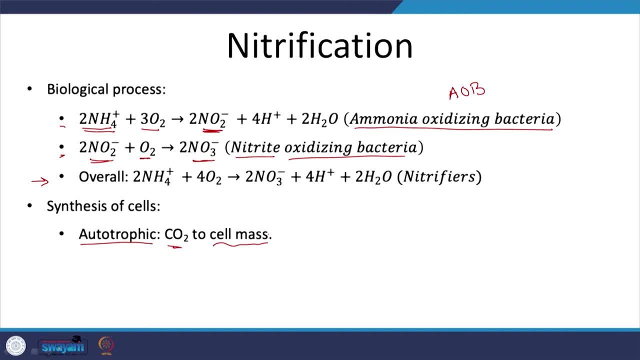 cell mass, for production of cell mass, but for the BOD removal, the kind of bacteria that are heterotrophs. So they need organic compounds for cell synthesis. we already looked at the relevant reaction. So what are the characteristics or how do you know? based on this, I can also 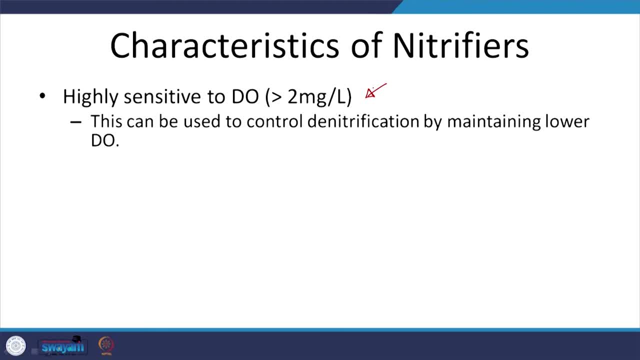 you know, figure out when to have nitrification taking place, and so on and so forth. So they are very sensitive to devo, as in only when the dissolved oxygen is high will this takes place, is it, I guess? so you need a lot of oxygen. 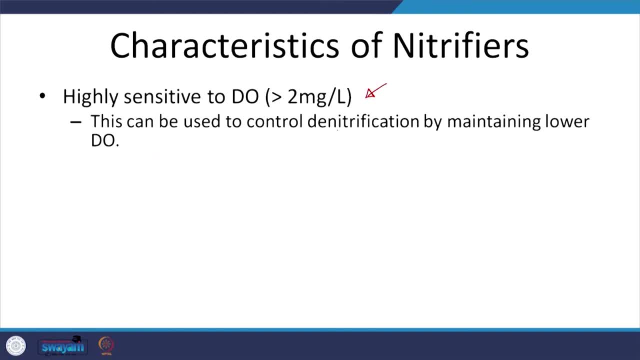 So dissolved oxygen has to be high. so if the dissolved oxygen levels are relatively low, this nitrification and then the subsequent denitrification will not occur. They are highly sensitive to toxics. So that is why, if you remember, in the BOD test we add denitrifiers, which more or less means 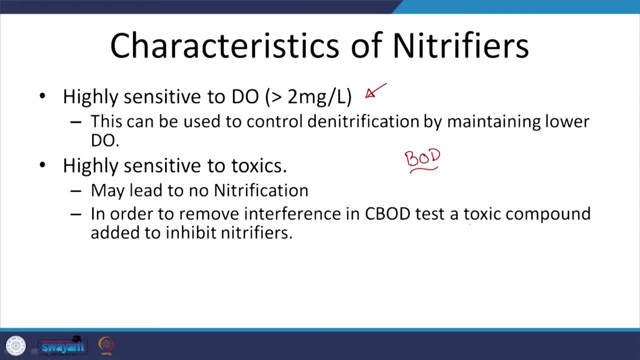 we are adding a compound that is specifically toxic to these nitrifying compounds, as in the ammonia oxidizing bacteria and nitrite oxidizing bacteria. So we add compounds that are toxic to this. that is something we do in the BOD test, but But again, they are highly sensitive to toxics compared to the other compounds. 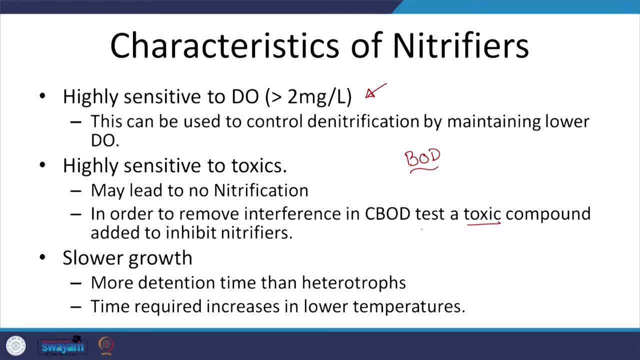 And they are slower, I guess growers, if I may say so. So more time is required than the heterotrophs which will do the job for organic compounds. So these compounds which look at NH4 and such, or the ammonia, they require more time. 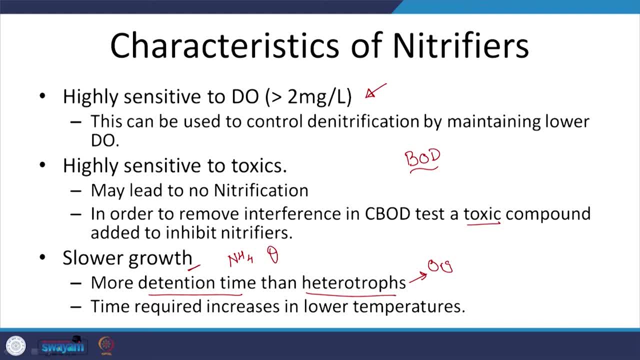 So HRT is typically high, So time required increases when lower temperatures. that is something that we already know. So in this case we looked at What is it now? nitrification, as in NH4 plus going to NO3 minus two half, two reactions. 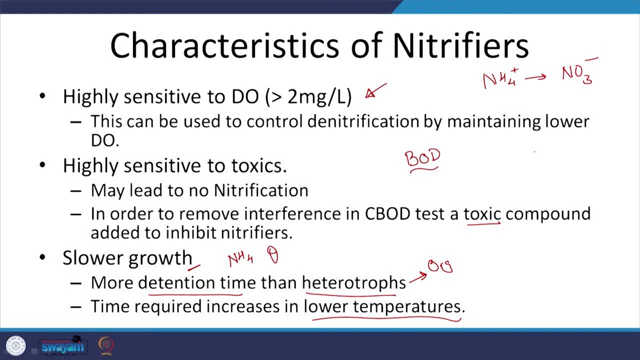 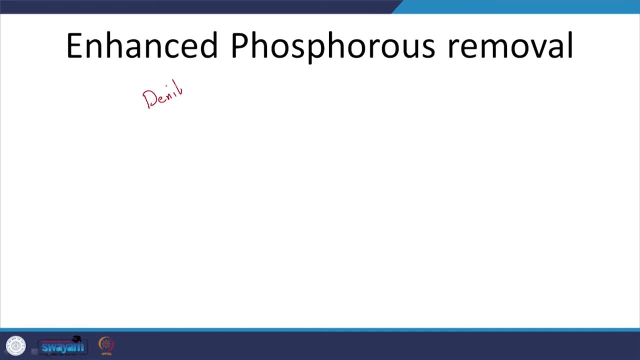 not half reactions, and then you will have denitrification. I guess I should have another slide here before enhanced phosphorus removal. So you have denitrification. So for that, what do you want? you need organic compound, You need an electron acceptor, which is what we are trying to remove: NO3 minus. 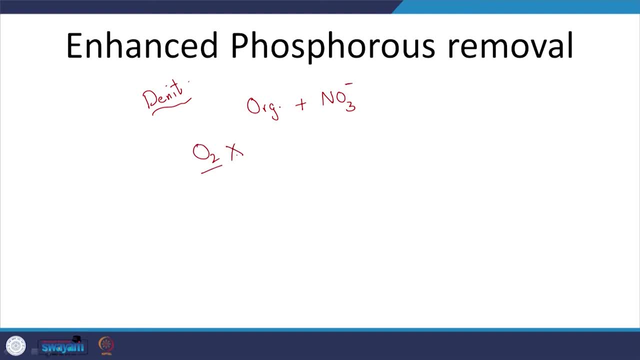 So here, if oxygen is present, this will not occur, So obligately anoxic. So that is one aspect. So oxygen is present, this will not occur, And then you need some phosphorus And then you are going to have the relevant reaction going through. 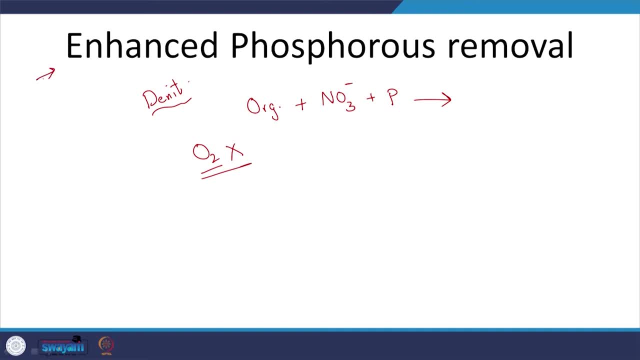 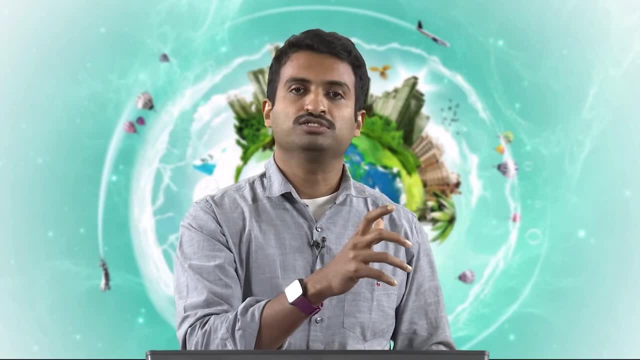 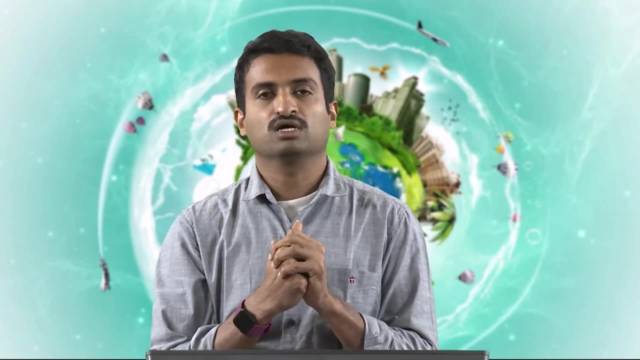 Similarly, for what is it enhanced phosphorus removal? Well, I guess, typically phosphorus is accumulated by a certain kind of microbes. So you are going to create conditions such that you have these microbes thriving and the phosphorus is accumulated in these relevant Compounds and then they are degraded. 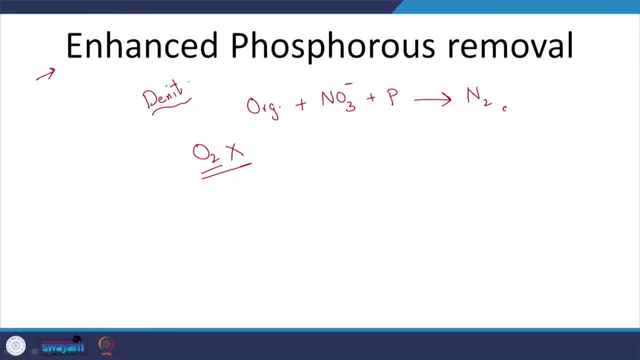 So what do we have with respect to denitrification? I guess nitrogen gas is formed. So for enhanced phosphorus removal, we are trying to achieve accumulation of around 8%, But this we will discuss later. There are certain conditions you need to maintain for these phosphorus accumulating bacteria to 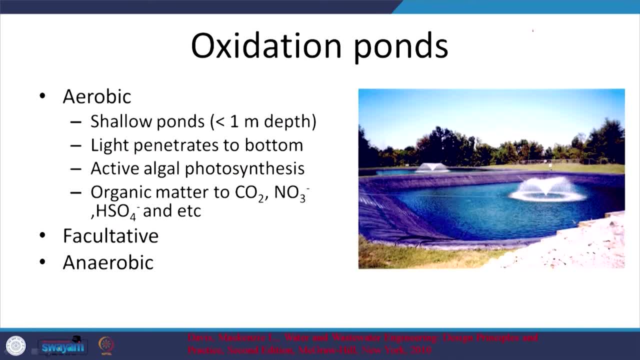 thrive. So let us move on. So we discussed activated sludge process in some detail, Only some detail. we will come back to that. But let us also look at the different, what we say- treatment mechanisms which are sometimes still used in the western world or were used in India. 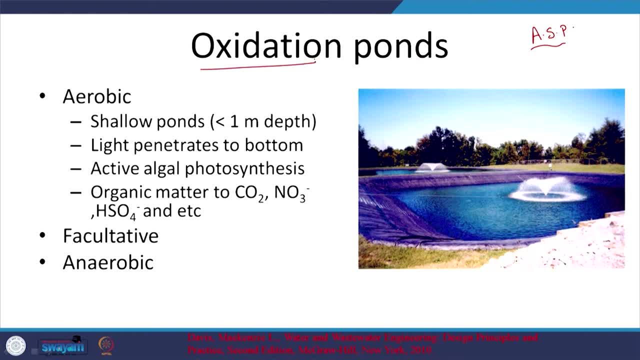 So oxidation ponds, Again oxidation, So you will have a source of oxygen. that is why oxidation. But they are shallow. Why, if not shallow? you are going to have anaerobic conditions, as in no oxygen conditions at the bottom. And here light penetrates to the bottom because it is shallow too. 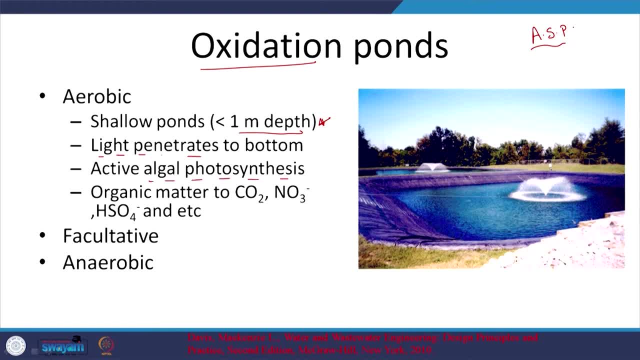 And then you are going to have Algal photosynthesis that will lead to your presence of, or generation of, oxygen- Algae photosynthesis- and you are going to have presence of oxygen And around this algal system you will also have bacteria which will use this oxygen. 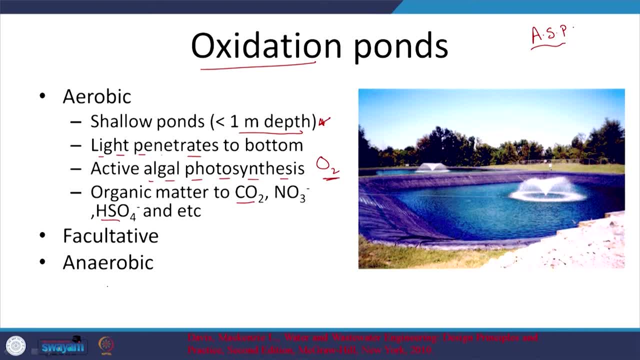 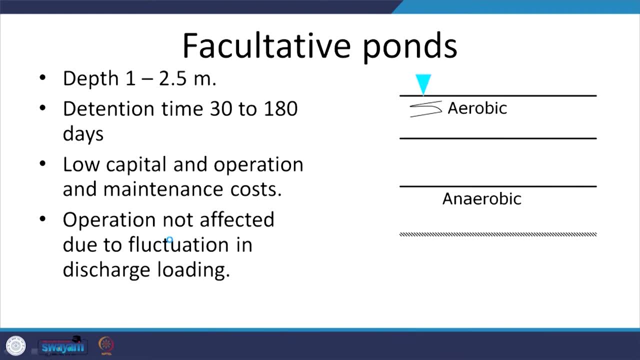 And then degrade the organic matter to the relevant byproducts. So, depending upon the size, you can have what do we say? faculty 2 and anaerobic zones? I think we are going to discuss this. If I increase the depth, let us say 2.5, 3 meters. 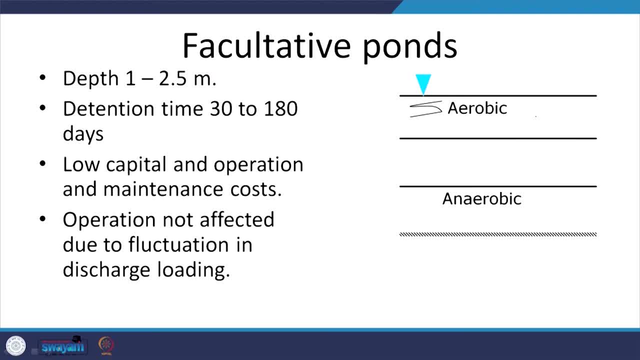 What am I going to have? The light is not going to penetrate to the bottom, So I will only have oxygen generation here. So aerobic conditions. here At the bottom, it will be anaerobic conditions, No oxygen, let us see. So I am going to have anaerobic conditions at the bottom. 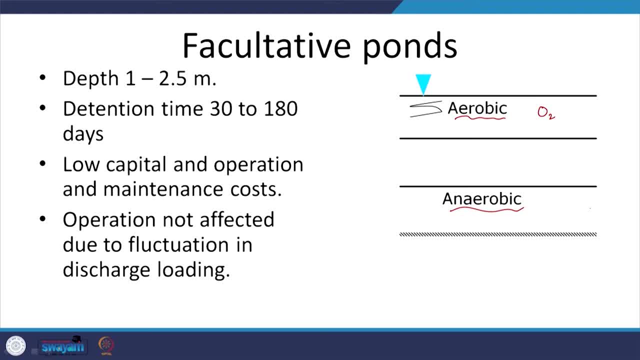 Different kinds of microbes will thrive here. But again, there is a symbiosis between these three layers, But we are not going to go into that detail here Here. but obviously, why will people choose this? Again, here you are going to have faculty 2.. 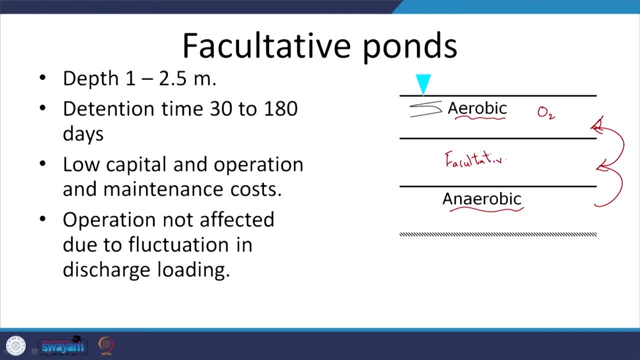 Those that can, I guess, more or less do both. Let us see, if I may say so, Why will people choose this? As you can see here, you are not providing oxygen, So it is cheap. But why would not you choose this, especially in India? 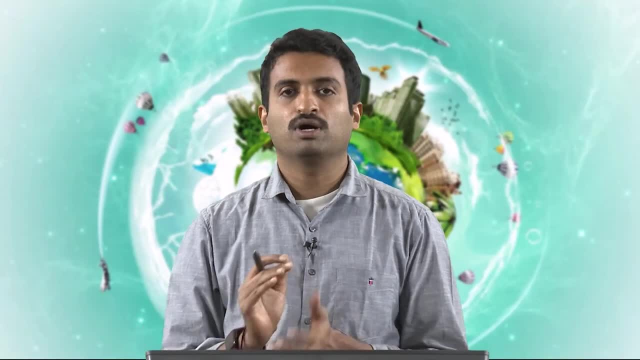 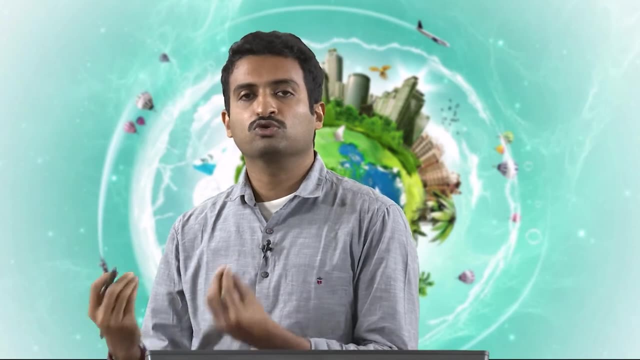 Well, we do not have as much land, And also water is a much precious resource here in India. And then, if you have relatively less removal efficiency, You are not going to be able to use your relevant wastewater Because, again, the nature cannot degrade your effluent. 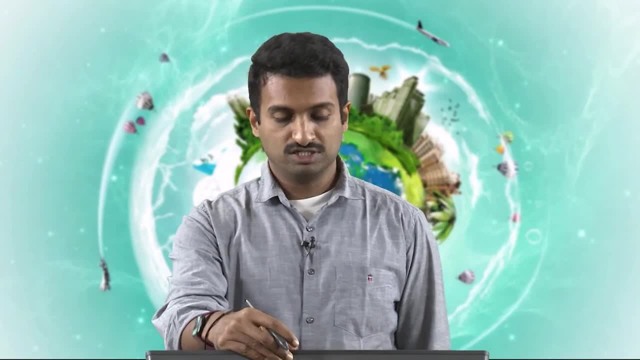 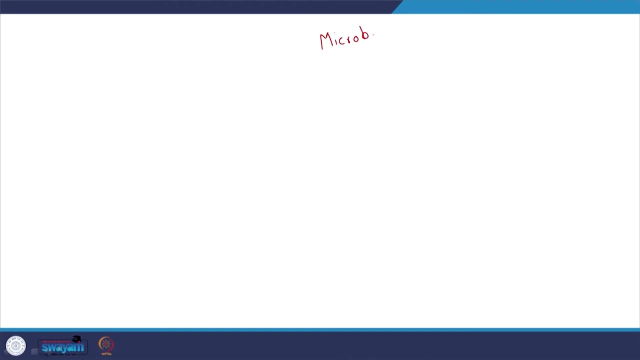 Let us see, Right. So that is one aspect to keep in mind. Let us see what else I have. So we are going to look at, I guess, microbes and how they grow. So the picture that we have here is that, if this is a closed system, 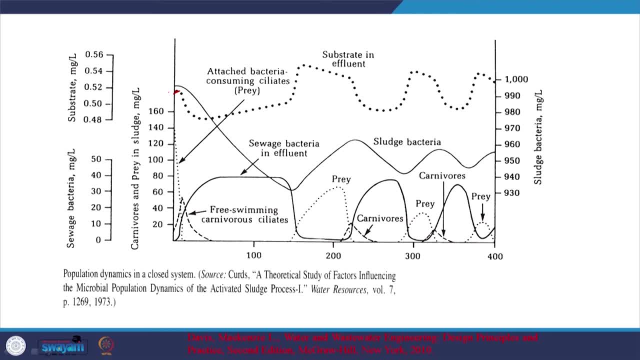 And I provide some substrate initially, Just maintain some substrate, Very low substrate. How is it going to? how is the system going to behave? So again, substrate. that is what we have. So we have sewage bacteria represented by this, represented by this, And then sludge bacteria, represented by this. 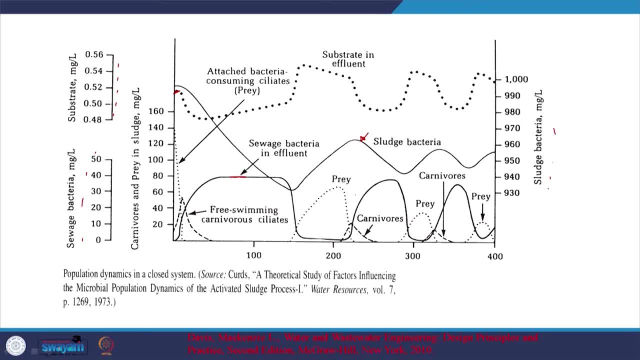 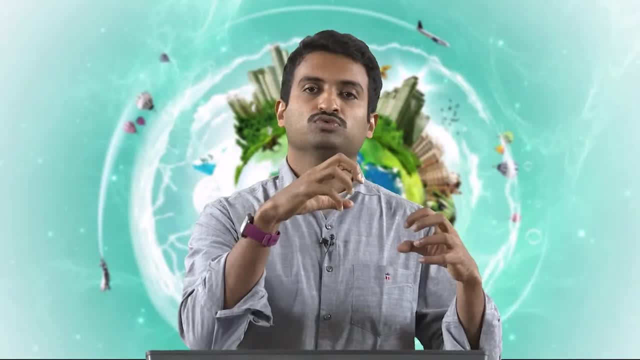 As you can see, at different times you will have different- what do we say? types of microorganisms thriving. Why is that? Let us say, once certain kinds of bacteria thrive, then you are going to have the carnivores which are going to feed on these kinds of bacteria. 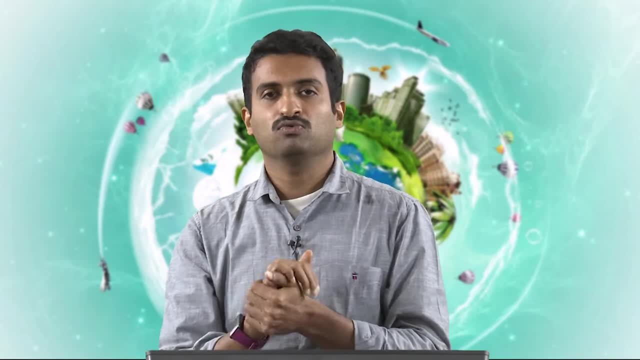 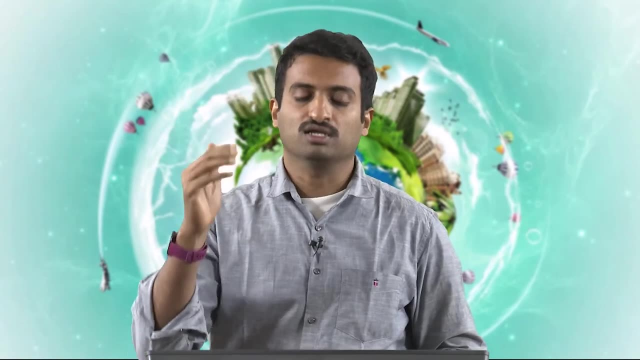 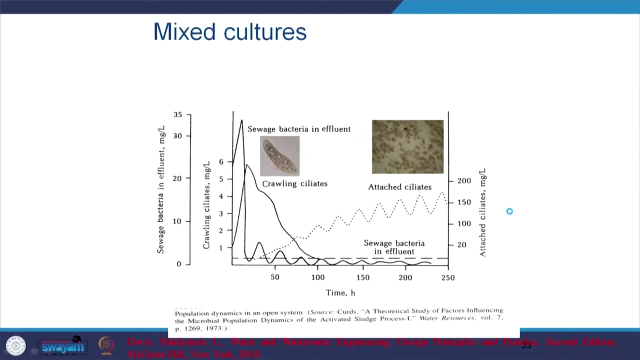 But when you do not have these bacteria which can feed the carnivores, Then the carnivores are going to die Again, then you will have have a different kind of bacteria growing, and so on and so forth. So it is cyclical. So that is what you can see out here. We are not going to go into detail here. Let us move on. 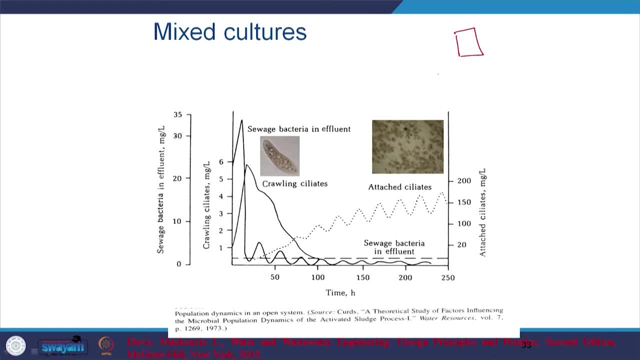 But in continuous flow systems. the earlier one was closer system, But here if it is continuous flow, as in what we experience in the wastewater treatment plants. So what do you see here? It is a dynamic system. Initially one kind of bacteria and then the different kind. 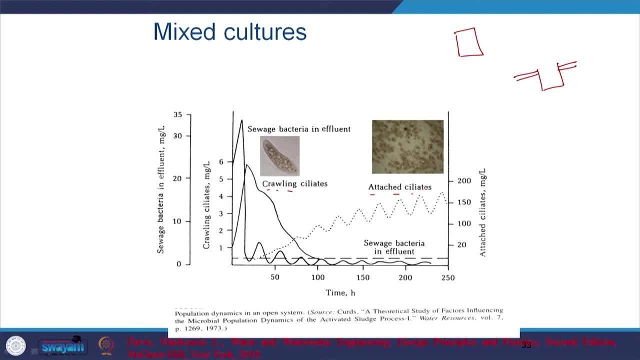 So here, as you can see, the system is pretty sensitive too, But over time you are going to try to achieve the kind of bacteria that will increase the efficiency of your relevant treatment process. So what do we have here? COH bacteria in the effluent. That is what we have here. 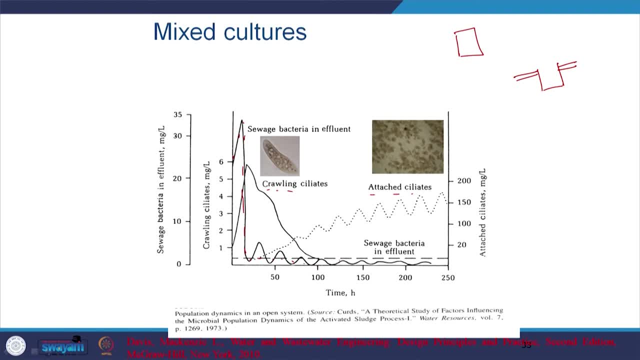 So that is going to decrease out here. Why? Because the kind of bacteria that are going to thrive in your aeration basin are going to eat up or not going to create conditions that are going to favor other kinds of bacteria, For example. one aspect I remember is that fungi. and bacteria which one will grow. It depends on which one has access to more food. Bacteria being smaller have greater surface area, So they can absorb the food faster, Not the case with fungi. So over time the bacteria are going to thrive. So that is what. 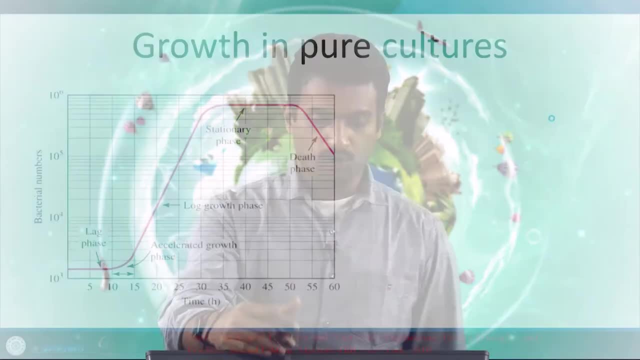 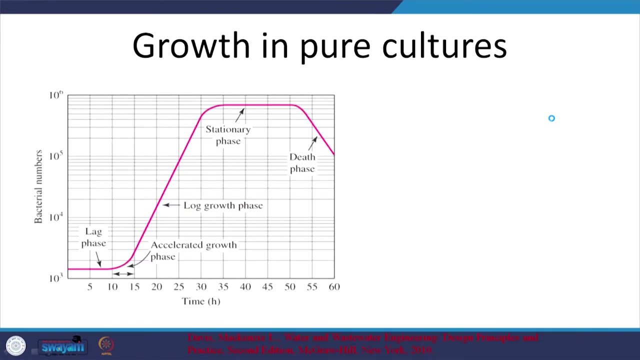 you are going to see, And that is one aspect to keep in mind. So how are they going to grow? We looked at one aspect here where we looked at it in detail, But if we look at a general case, I take a closed system. 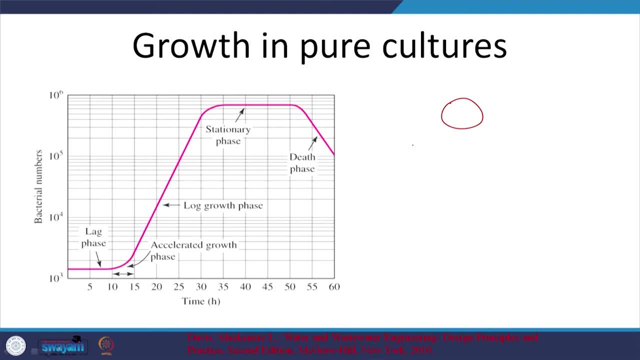 put some microbes and just look at the overall microbial growth. So in this graph let me also put in my substrate, or my food waste, my waste, which is the food for the microbes. So what is going to happen? Initially, we are going to have the lag phase On the y-axis. 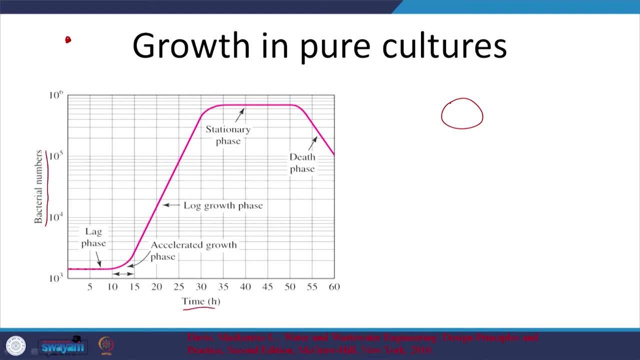 we have bacterial numbers On the x-axis: the time. Initially the bacteria get used to the relatively new environment. Initially the bacteria get used to the relatively new environment. So you are going to have lag phase. They are still getting used to the relevant environment. 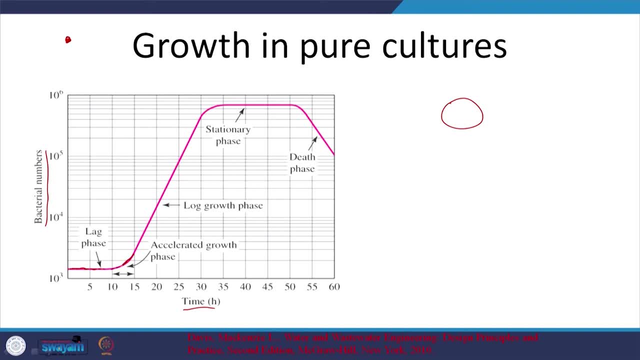 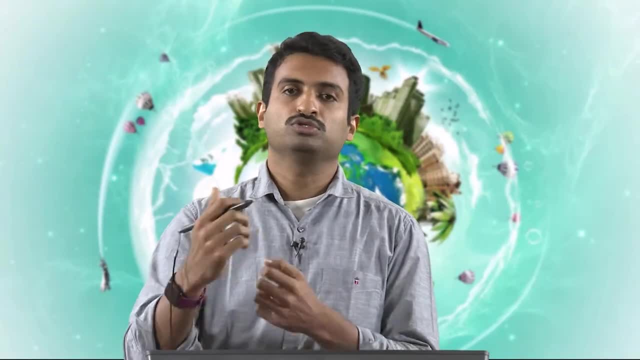 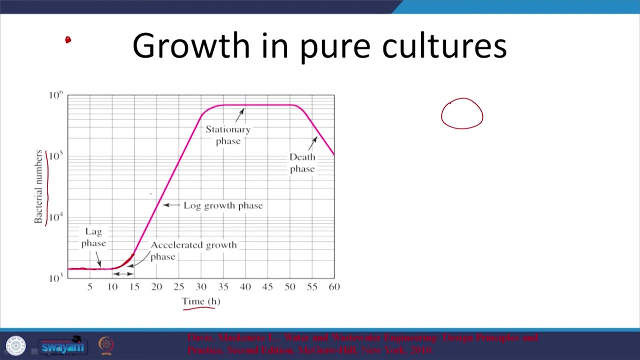 Once they are used to the environment. you are going to have an accelerated growth phase. Here. different bacteria are going to have different rates of growth, but they are going to start growing And then we are going to have log growth phase. As you can see, it is linear, So more or? 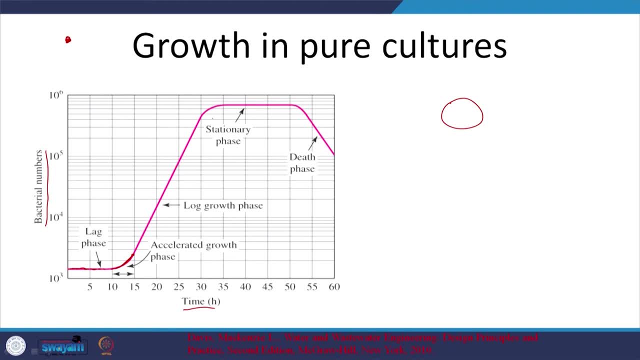 less. the growth rate is relatively uniform or a regular growth rate, And then stationary phase in this during this time. what is going to happen? All this time? your substrate or the food waste is going to come down. So at this point, as you can see, there is no more food for the 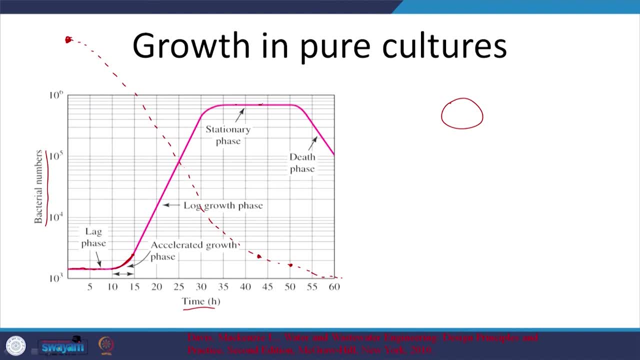 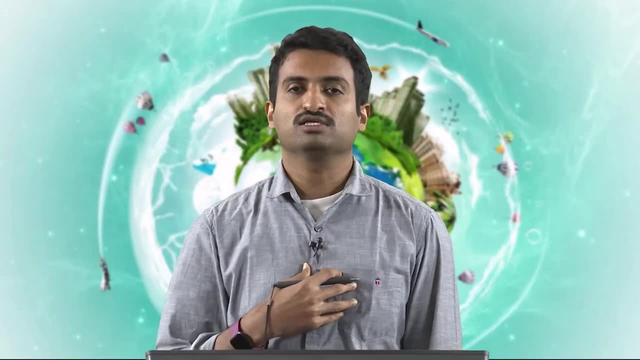 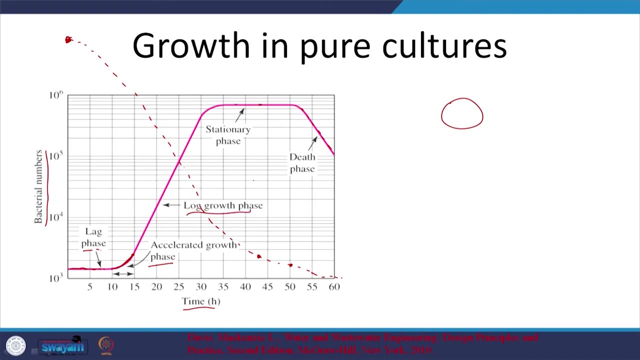 microbes, or maybe even here. So here the cell or dead cells itself are going to serve as food for the other microbes, And afterwards, you know, there you have nothing there, And then you have the death phase. I guess, right. So four phases: lag phase, accelerated growth, log growth. 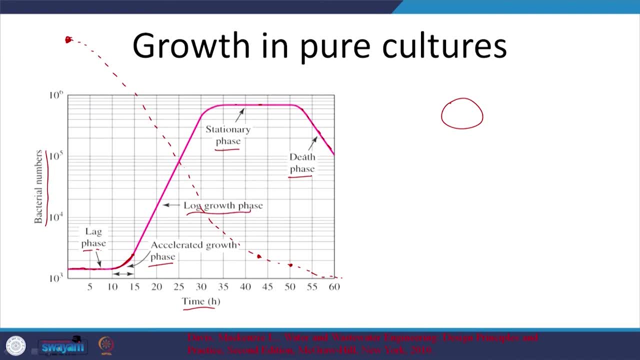 and stationary and, in general, death. but in a continuous flow system- you are going to try to see to it that you provide food continuously- there will be some decay, but that is a different aspect, let us see. So we are going to look at this log growth phase. So this is how bacteria 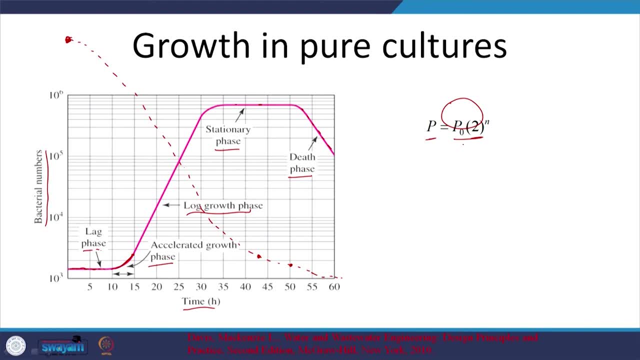 can, what do we say? grow? I believe we have a relevant numeric problem later. So, population, after what do we say? n? number of generations initial, what do we say? population as in one goes to 2,, 2 goes to 4.. So based on the generation time, you can calculate that. 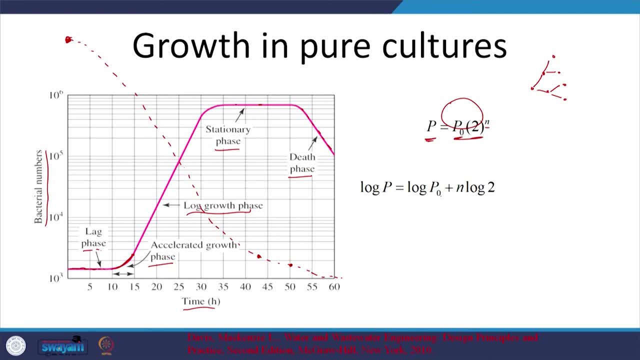 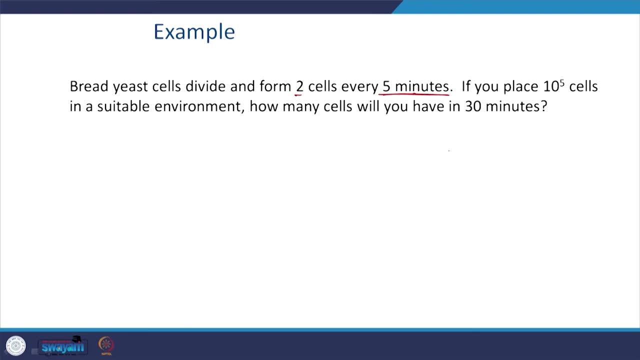 Let us see what we have. So log p equal to log p naught plus n log 2. So bred each cells, divide and form 2 cells every 5 minutes, 5 minutes generation time. So if I initially have 10 to 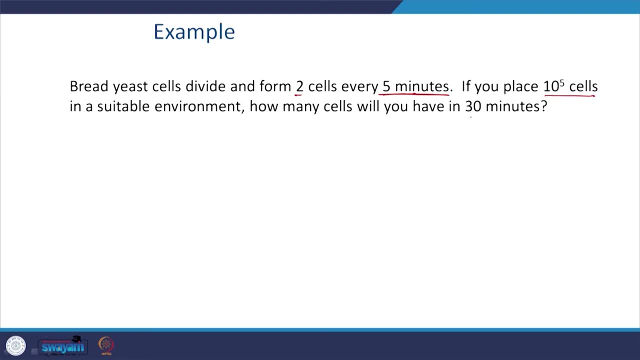 the power of 5 cells in a suitable environment. how many cells will I have in 30 minutes? So 6 generations out here, I guess. So 30 minutes by 5 minutes per generation, 6 generations. So p is equal to 10 power, 5 initial p naught into 2 to the power of n number of. 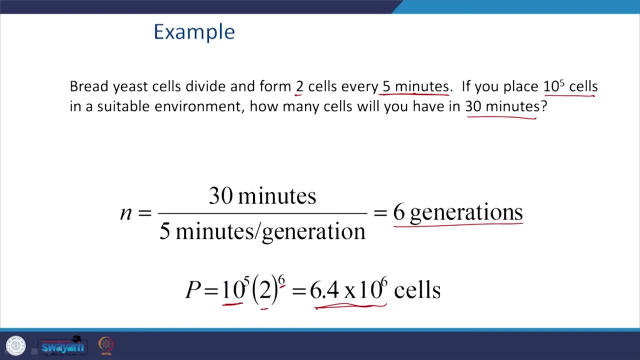 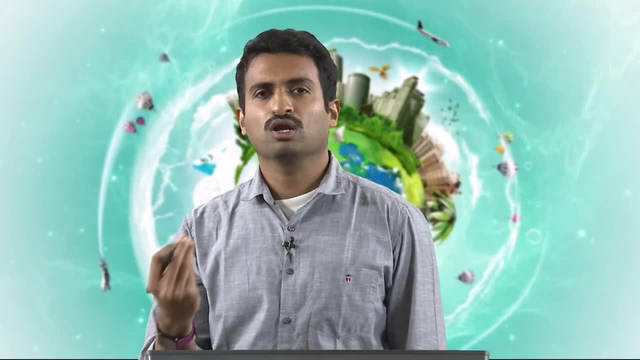 generations. So you see 10 power 5 end up to be 6.4 into 10 power 6 within 30 minutes. So they grow a lot. the mass will not increase, but they grow a lot. it is the numbers that count, not the. 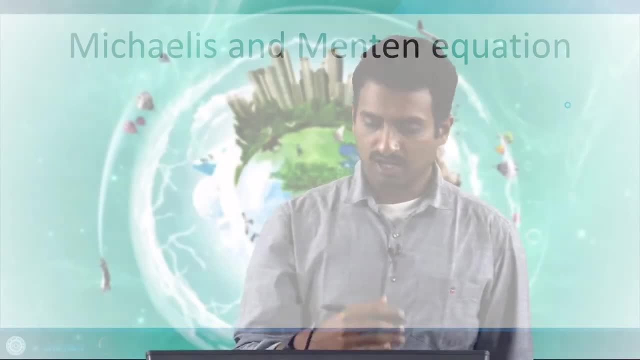 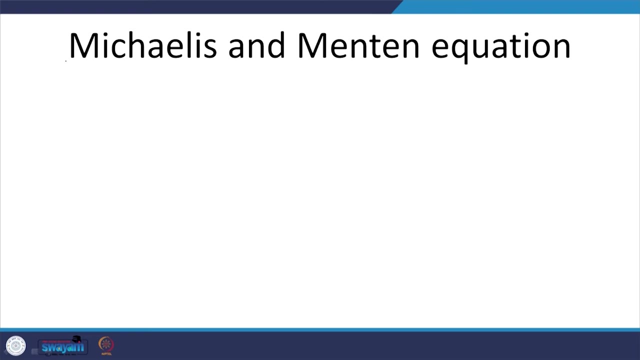 mass. So that is one aspect to note here. So how is it that the microbes degrade your relevant substrate or are waste? We are going to look at this particular equation, but we are not going to derive that. So what do we have? We have enzyme and the substrate, enzyme and substrate, And then you are going to have 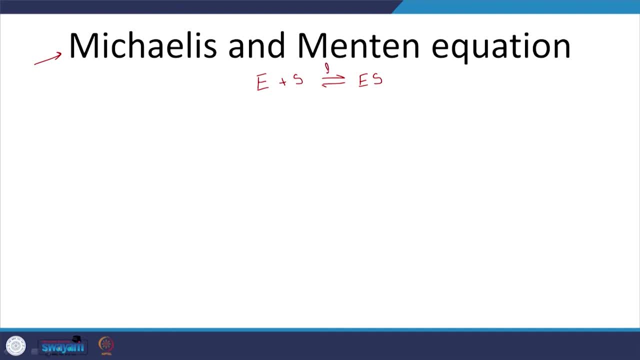 an intermediate product. Yes, So K1, K2, forward reaction, backward reaction, And then this will go to the products K3.. Yes, this is what you have And the rate of production of this products or such. you can get it by applying this mass balance on this particular what is it Es? 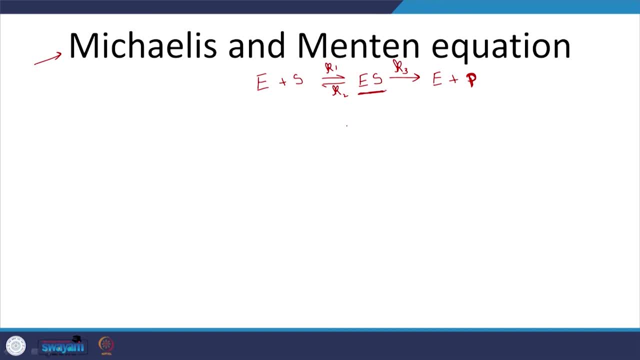 And then you can get it. And it is just looking at the reactions that lead to formation. So what are leading to formation? K1. I mean E plus S is leading to formation And the backward reaction is leading to loss. And 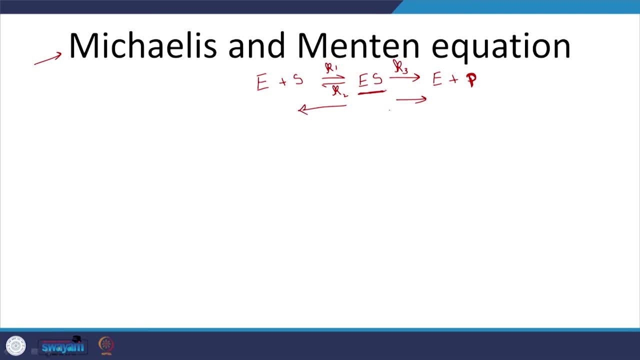 this reaction also is leading to loss. So you can apply mass balance and get it, But we are not going to do that here. But more or less, if I am not wrong, R will be going to be equal to R max into S by K plus. yes, S is the substrate concentration And K, I guess, is nothing but. 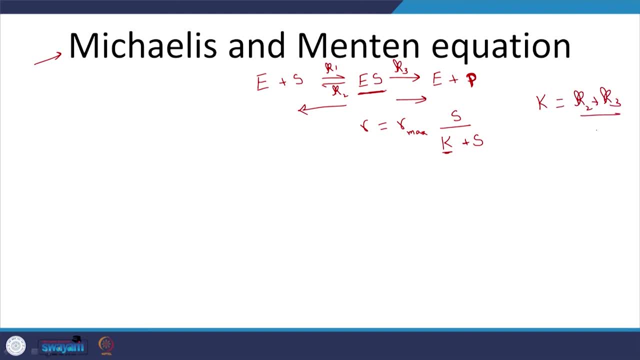 equal to K2 plus K3 by K1.. Again, you can look at the relevant derivation. So what does that tell us? What will the profile look like if this is R and if this is substrate? So the profile will look like something like this, And at this point it is S, when the S is high, And here, I guess, is. 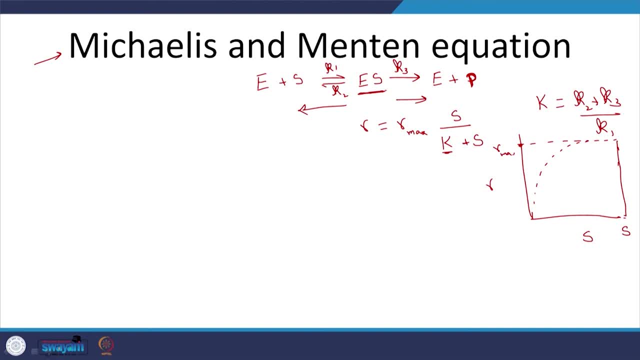 R max. R max. At this point, R is R max, As in when S is far greater than K. what do you see? S? S cancel out and R equal to R max. So that is what we have, And also I am the case when it is. 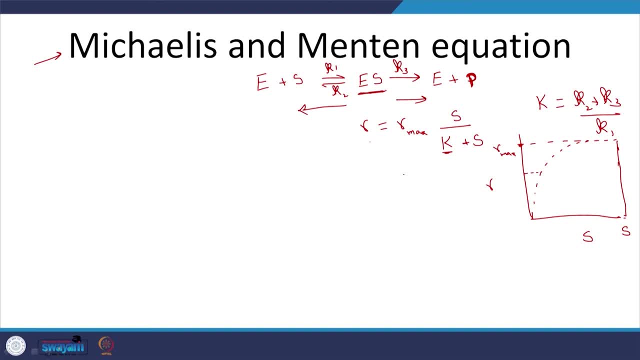 at half. I guess when S is equal to KS, you can think of that. Then it will be R max by 2 KS. I guess us is the Michaelis-Menten equation Similar to this. people observed that, or Mr Mano? 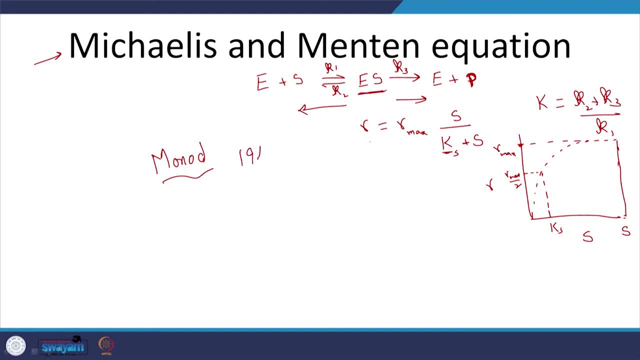 or Dr Mano observed that I think it was in 1949.. The microbes also have a similar profile, profile for growth- and that is what we are going to look at. The profile is similar to this: R equal to R, max to S by KS plus S. This is a constant, as you can see, and S. 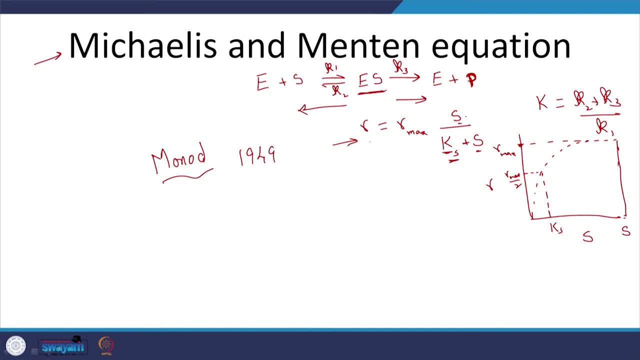 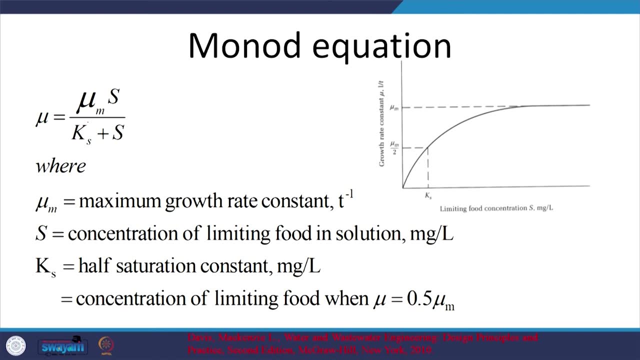 is the substrate, One aspect to keep in mind. we will just discuss this later. What do we have? Let us see. Mano equation, as you can see, is similar to this. Let us look at what the variables are here. This is the specific growth rate: different names. 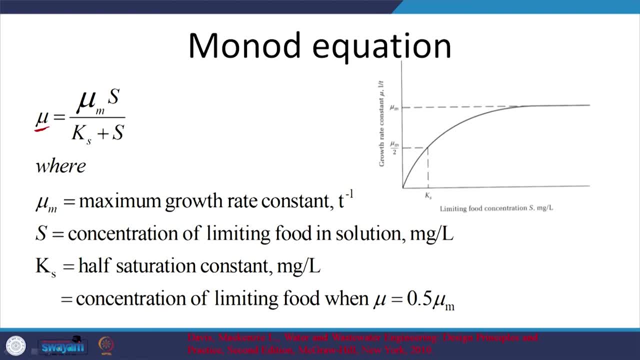 You can look at that specific growth rate and such. Here mu max similar to R is equal to R max into S by K plus S. I think earlier it was KM and now it is called KS. Here you have mu specific growth rate. Here mu max is equal to mu max into S by KS plus S. Earlier it is KM, here it is KS. 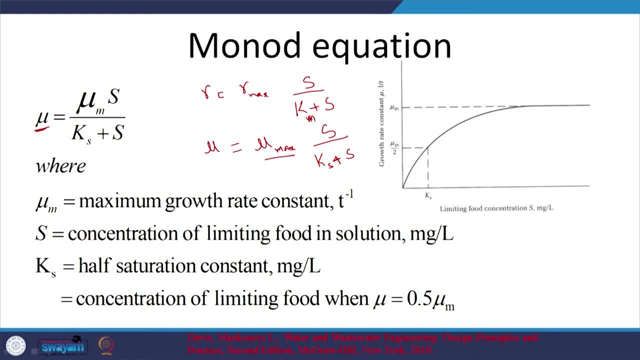 What is this maximum? It is maximum growth rate constant of the microbes. This will tell me the new cells, mass of new cells per the cells existing already, per time. These two cancel out and that is why units are per time, But they are more or less giving me an idea. 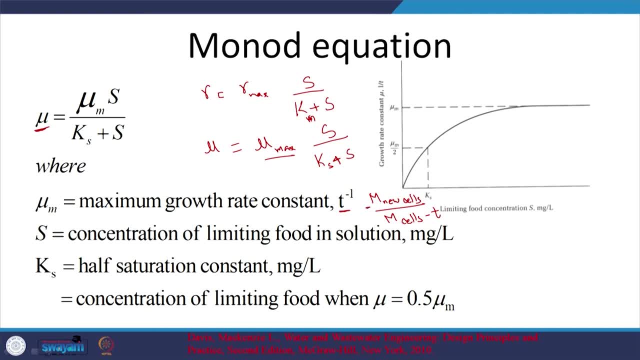 about how much new cells are being generated per the existing cells per time, And S is the concentration of the food for the microbes or our waste. That is what we have. KS is the half saturation constant. when will the mu max be half? That is what 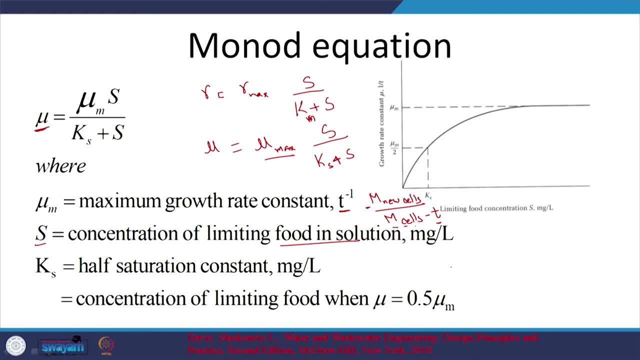 we have And what else do I have here? Half saturation, constant concentration of limiting food when mu is equal to 0.5 mu. That is something you have. You can plug that in And see that out here. Let us see that mu is equal to mu max into S by KS plus S. This. 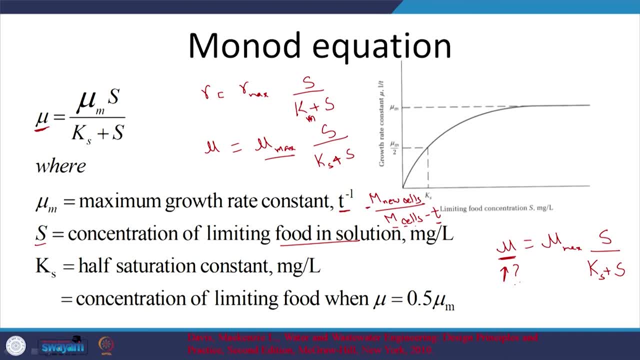 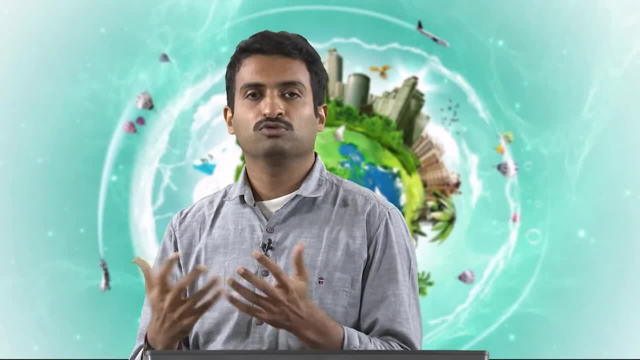 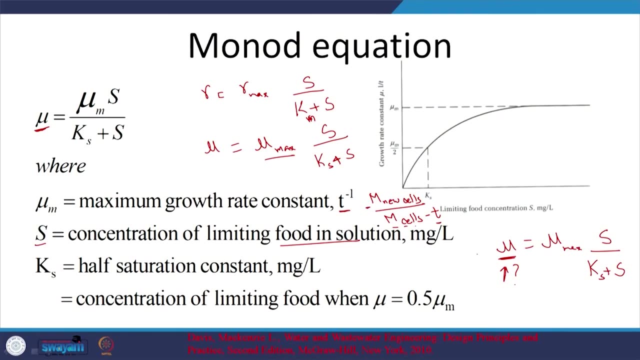 is going to give me an idea about why is this important? now I want to know how cells are growing or how the microbes are growing. So this is what will give me an idea about how the microbes are growing. So, as was observed by Mr Manu, and that is why we are calling that the Manu equation- We have the specific 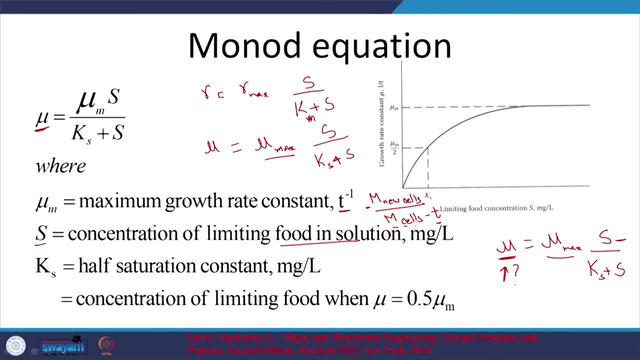 growth rate being depend upon the maximum The food and this relevant constant out here, And I was just trying to say: when will this be the case? Let me just look at that. So you want: KS is when mu max is equal to half. 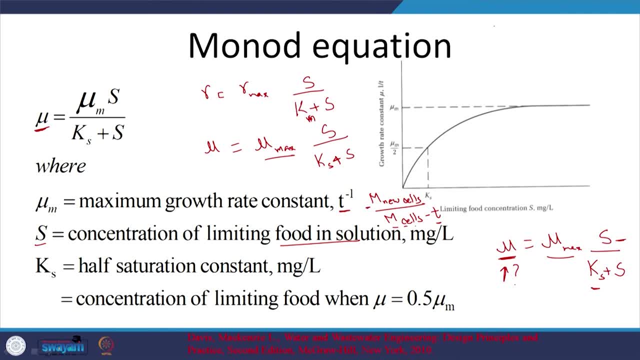 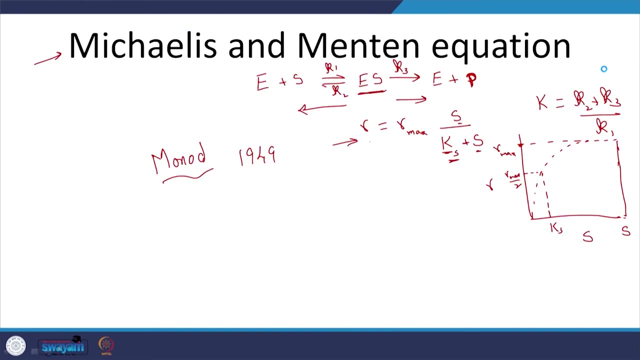 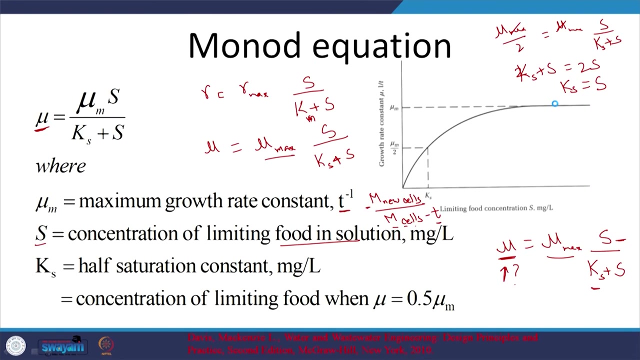 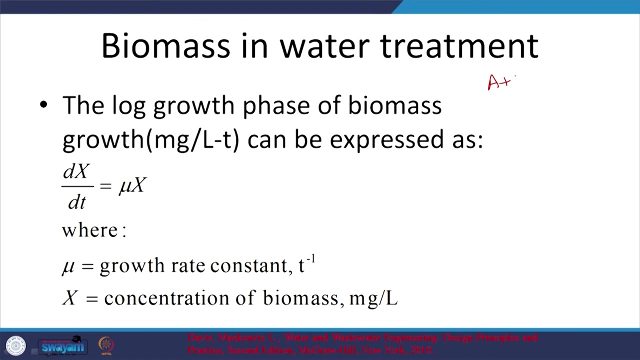 In which conditions will that turn out to be? If this is, mu max by 2 is equal to mu max S by KS plus S. So that is your rate of growth of the relevant microbes. Let us move on Manu equation there. 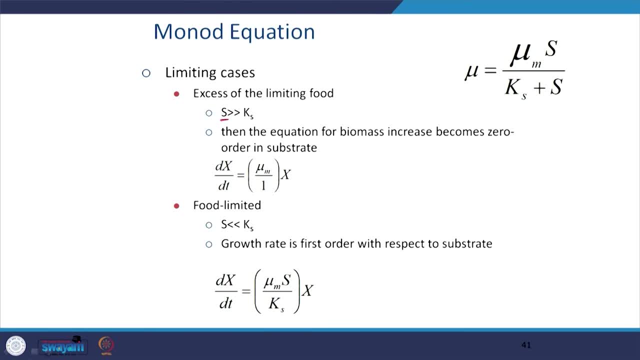 are limiting cases here. One is: when we have a lot of food, S is far greater than what we say KS. So when there is a lot of food, obviously you know the food is no more a limiting factor for the microbes. It is not dependent upon the relevant. what is that? 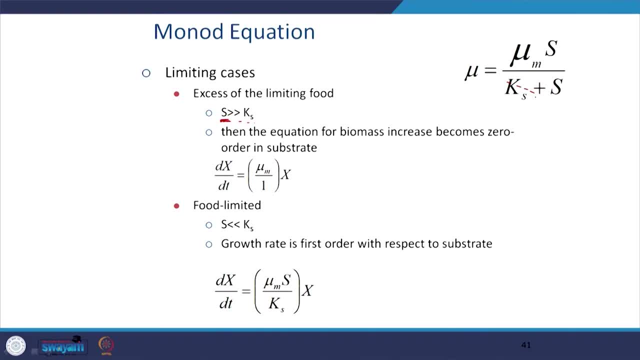 KS. When S is far greater than KS, we can neglect KS and then SS cancel out. Then mu becomes mu maximum. that is what we have out here. So it is only depend upon the amount of cells. but if food is less, if food is less, say F, it is far less than or S is far less. 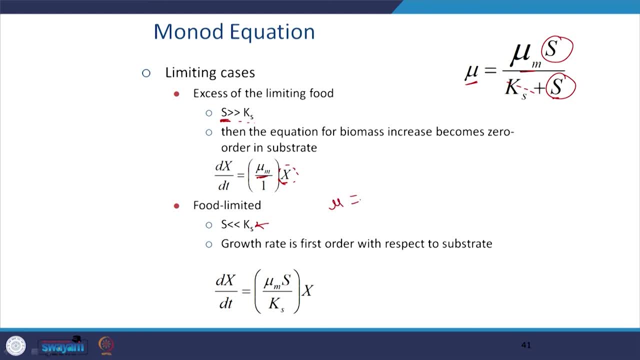 than Ks. So what is going to happen? mu is going to be equal to mu, max into S by Ks. So it is then very much dependent upon the food, and it is first order. that is what we see, and these are the two limiting cases out here. 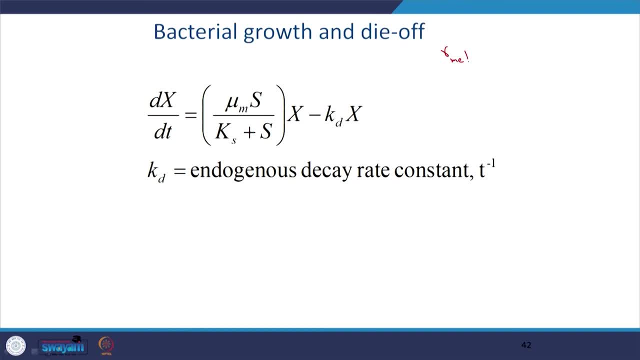 So bacterial growth, as we saw our R net. R net is going to be depend upon rate of growth of the bacteria and also rate of decay or death of the bacteria. So here we already developed the equation for rate of growth, which was equal to mu times X. that is what 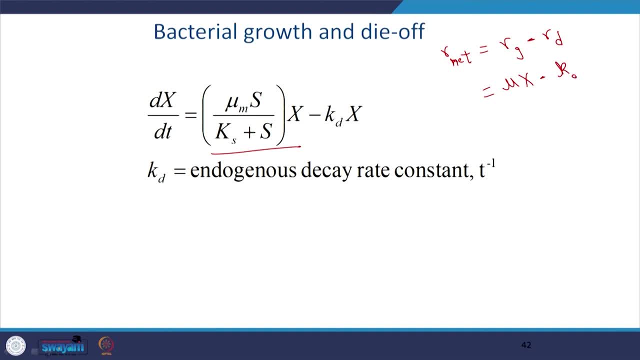 we have out here and death, that will also have a rate constant decay- endogenous decay. rate constant into the concentration. So that is what we have. this is the R net. So that is what we have. this is the R net. So that is what we have. this is the R net. 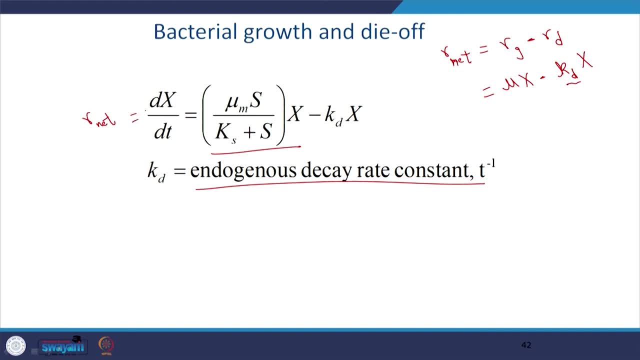 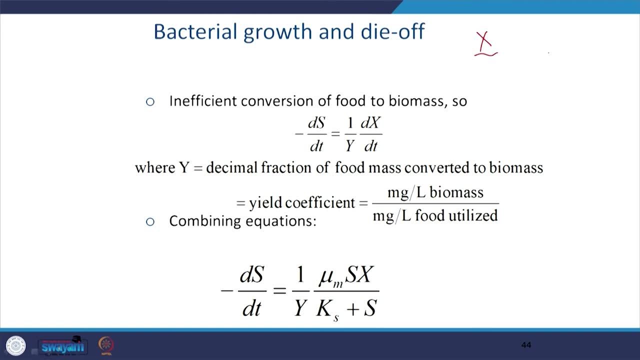 Considering the bacterial growth and the death. So let us move on. So, bacterial growth and death. So why am I concerned with this bacteria? at the end of the day, I am not here to feel philanthropic and have a lot of bacteria. It is because I want to degrade the waste. 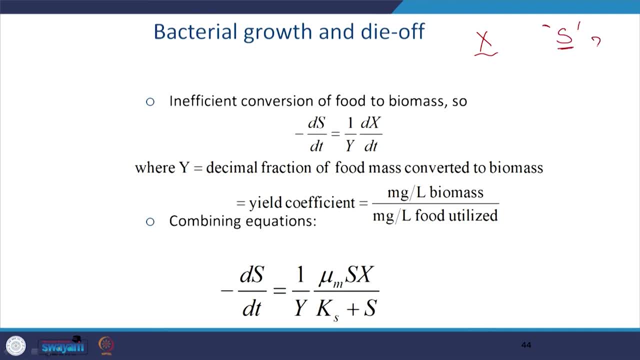 which I am representing by S. but what is S going to be depend upon? as we know, it is going to be depend upon how many bacteria are there. So the rate of removal of S will depend upon the rate of decay. So the rate of removal of S will depend upon the rate of decay. So 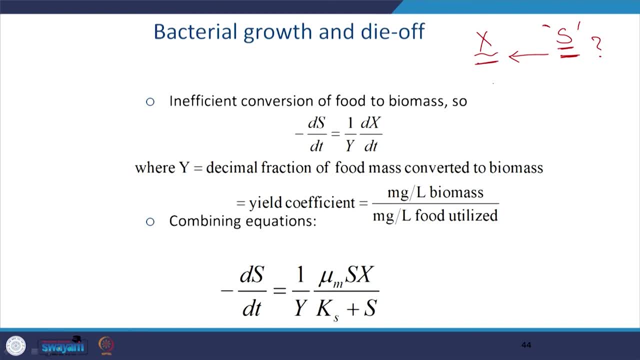 the rate of removal of S will depend upon the rate of decay, So the rate of growth of the relevant bacteria. So here we have two aspects. So rate of growth of what do we say? rate of growth of the microbes will be related to the rate of loss of the substrates. But both are not going to be the 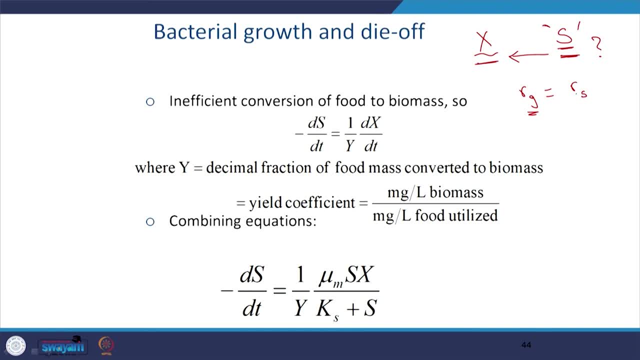 same. why is that? it is not so efficient? the process is not so efficient. you have relevant electron transfer and such. There are other aspects, So it is not going to be as efficient. So that is why you are going to have a variable here, which we call the yield coefficient. What is the yield coefficient going to give? 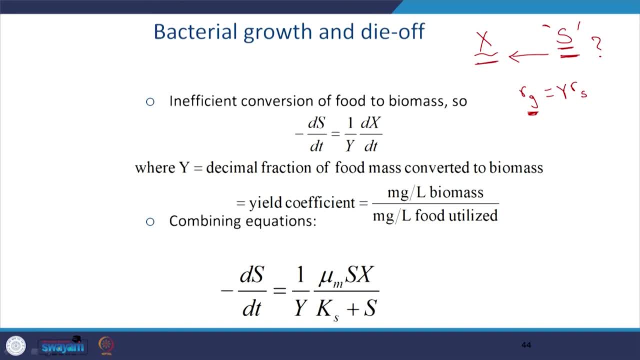 you an idea about? let me see if I have that. So here they are representing: occurs by ds, by dt, negative because it is being lost. rate of growth of microbes: dx by dt And 1 by y. they are bringing it out here, right? So rate of growth of microbes, we are going. 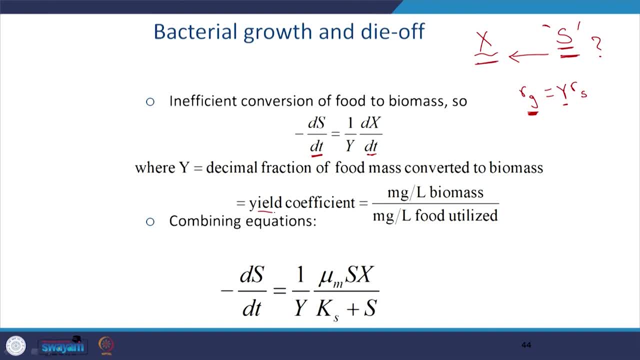 to have a fraction out here. What is this fraction called? it is called the yield coefficient: decimal fraction of food, mass food that is converted to food converted to biomass. As we know, not everything will be converted. Some of it will be used up for energy and such. 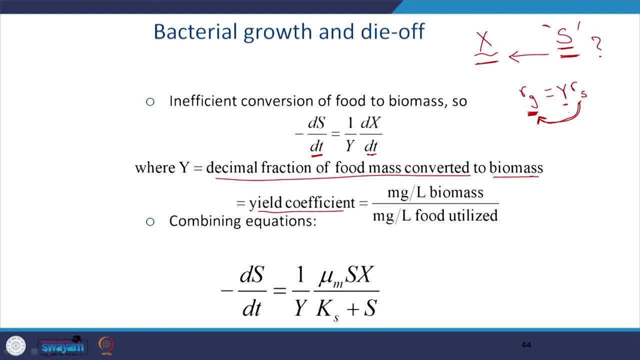 only some will be coming be used up for or converted to cell synthesis or for cell synthesis. So that is why you have this less than one yield coefficient. So this yield coefficient is nothing but milligrams of biomass for the milligrams of food utilized. So that is what you see out here. 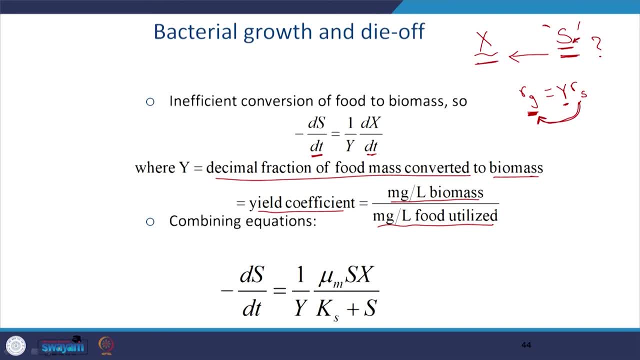 So from here I can calculate how much my the rate of my loss of substrate is. So rate of substrate loss is equal to 1 by y rate of growth of the relevant microbes and negative because it is being lost. So what do I have? I know that minus 1 by y into, depending on what equation you are using. 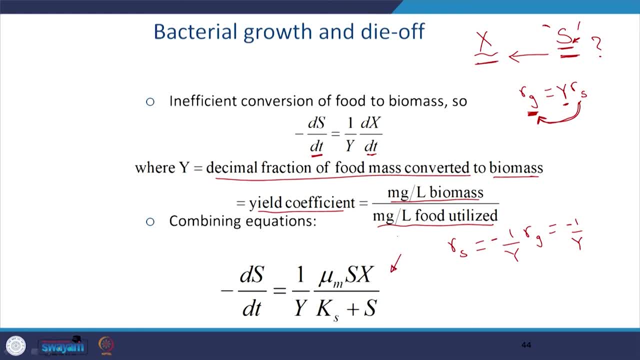 you will have this So dx by dt. we already looked at that there. So rate of growth of the relevant microbes, which is nothing but mu times x. So mu times x. what is mu Mu is mu max into s by k s plus s. 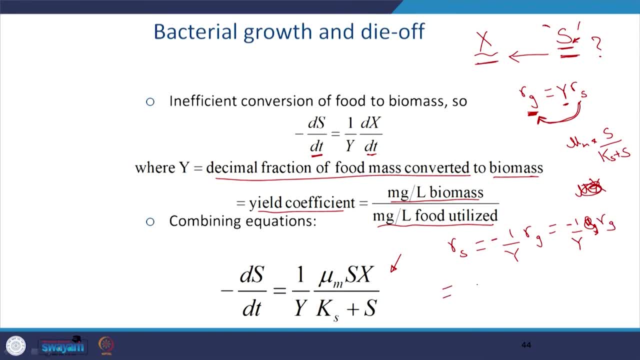 So rate of growth that is equal to minus mu times x by y, and because we know that mu is equal to this particular equation, we end up here. So that is what we see. You do not need to mug anything up. let me just summarize and end this session for today. So what are we trying to do? I am trying to understand. 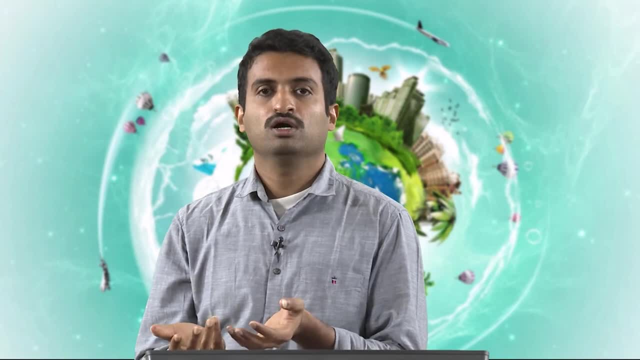 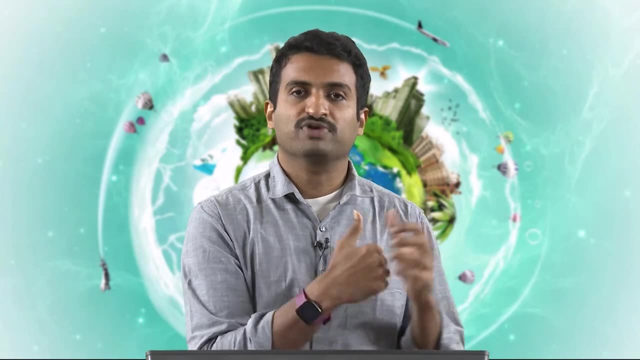 how microbes grow and what is the equation that tells you about it? It is the Mono equation, and what is this depend upon? It tells you, or what is it depend upon? this growth rate or specific growth rate, which we are saying is a constant. It depends upon. 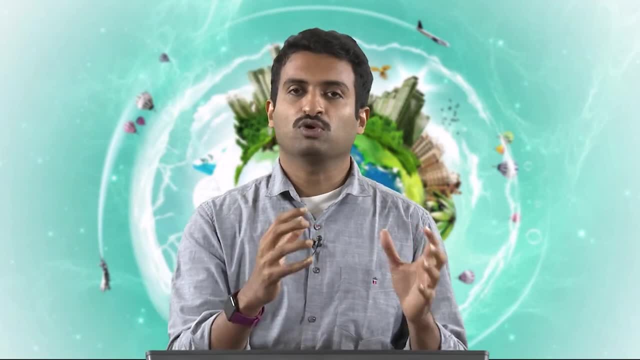 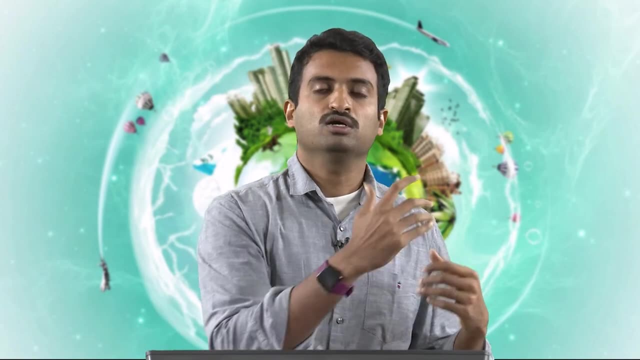 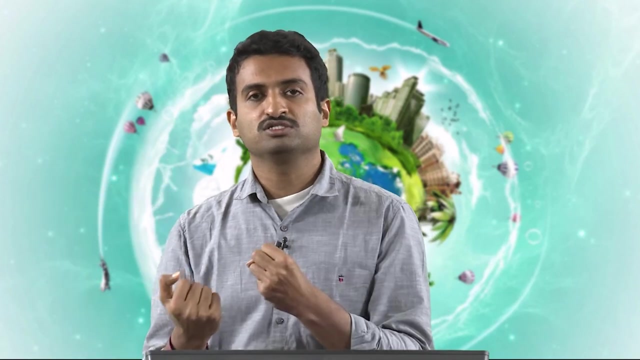 the substrate. how much food is there? So that is what we know, which is nothing but mu, max into s by ks plus s, and from that we can calculate how the microbes are growing. rate of growth. Why is that important? Because we know that the microbes grow by breaking down our waste. 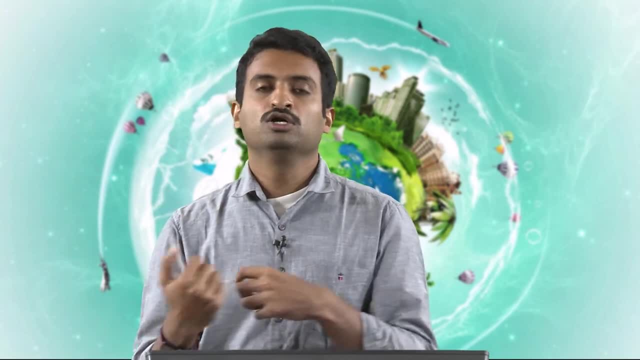 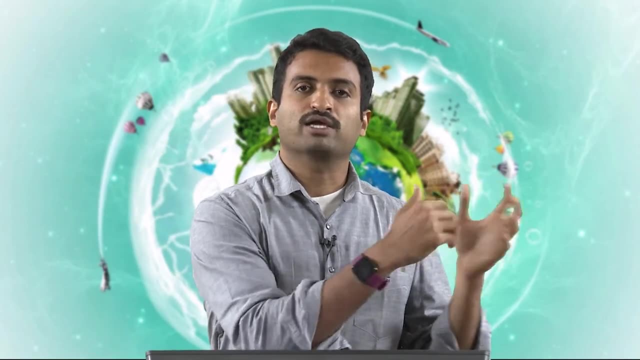 So we can relate our waste loss to the rate of growth of the microbes. but not all the waste that is being degraded will turn into the cells of the relevant microbes. So you are going to have to have a fraction that is called y, or the yield coefficient.